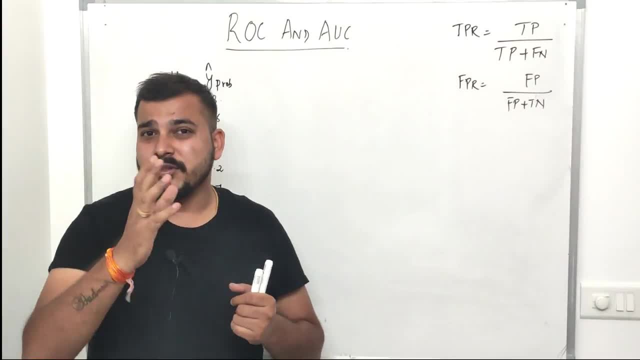 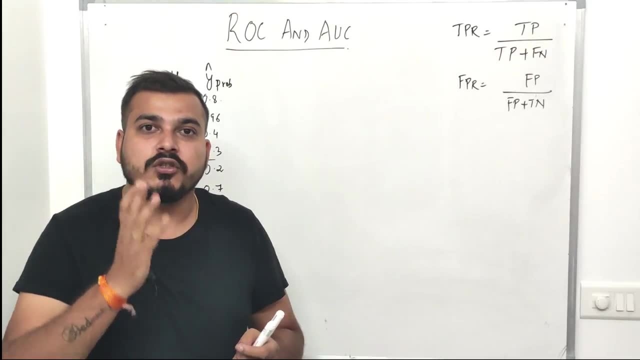 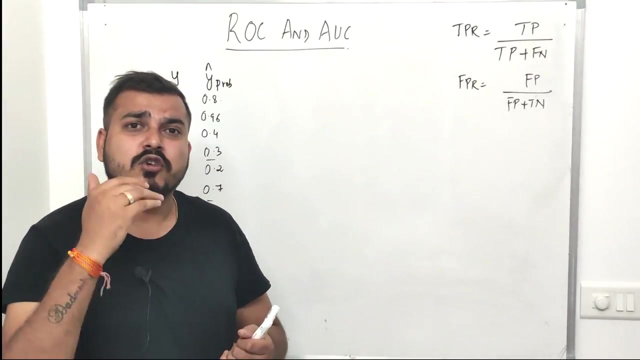 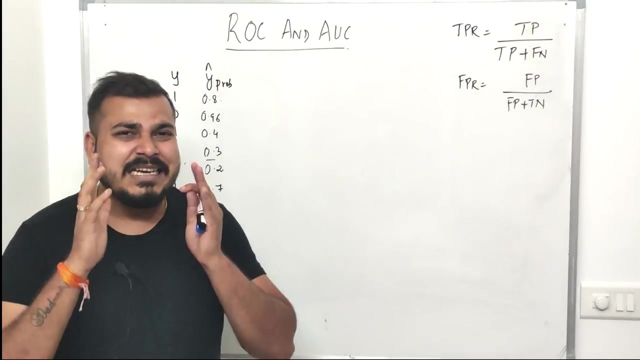 It is pretty much important that, suppose, if you are implementing a logistic regression and suppose your model has predicted some probabilities, So what is the threshold that you should decide so that, by default, if I consider logistic regression, it considers anything greater than 0.5, it is going to consider it as 1.. Anything less than 0.5, it is going to consider it as 0.. Now, understand one thing is that in each and every use case that you have, this threshold can play a very, very important role. 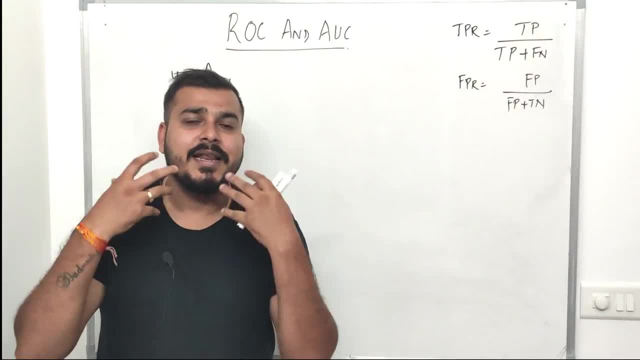 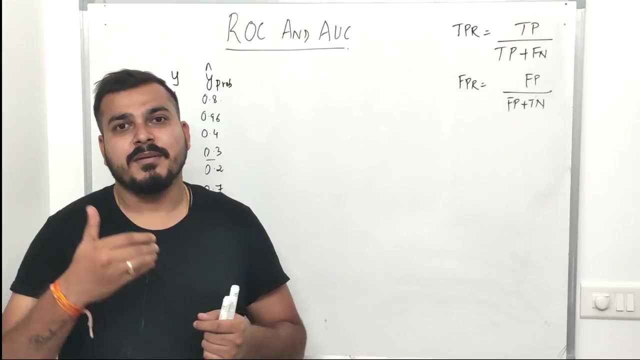 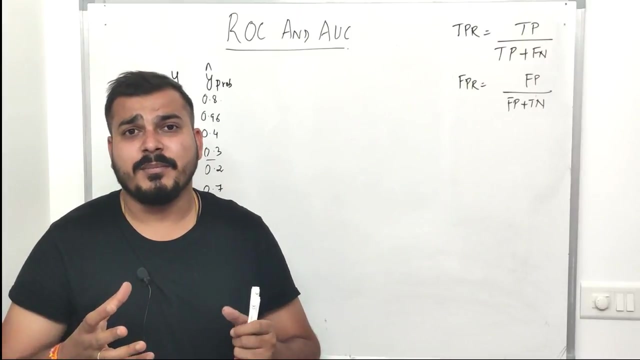 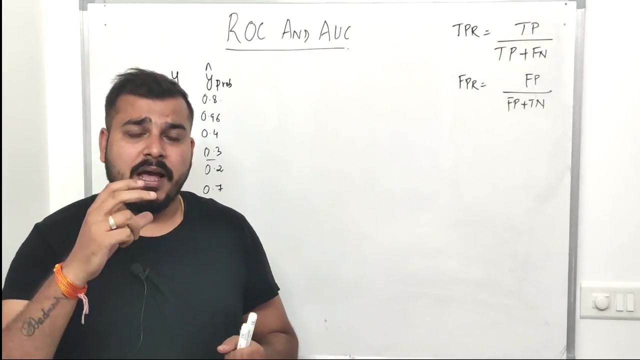 Now let me just take some examples about it. Suppose you are working in a healthcare domain project and the model that it is predicting it is very, very critical. You know it may be a disease patient, it may be something. So at that time you know what may happen- is that the threshold value that should be kept, based on the type of problem statement. Suppose you want higher true positive rate, you want less false positive rate. So based on that, we can actually play with the threshold and again, a domain expert person will always be there, will be able to guide you out. But remember, guys, you need to 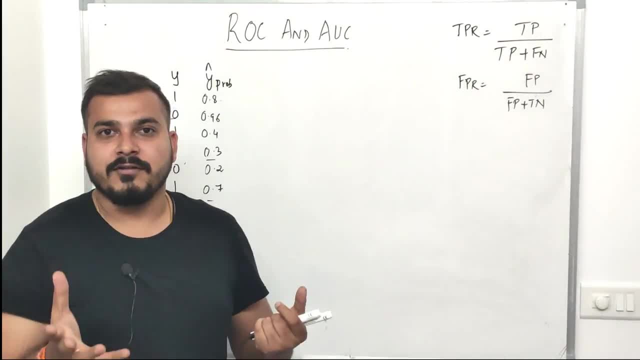 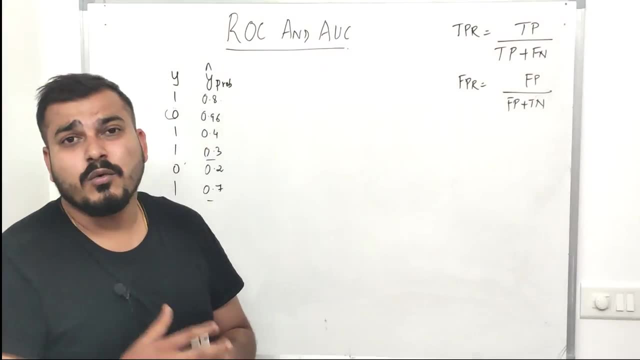 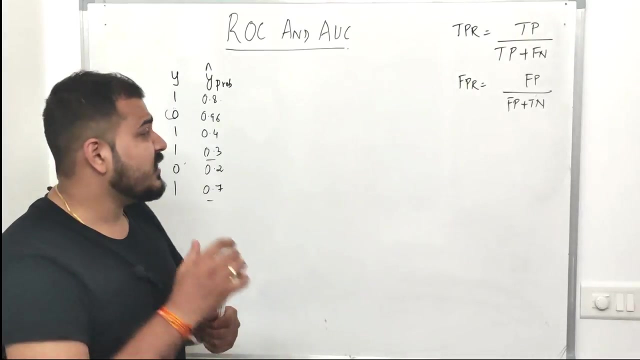 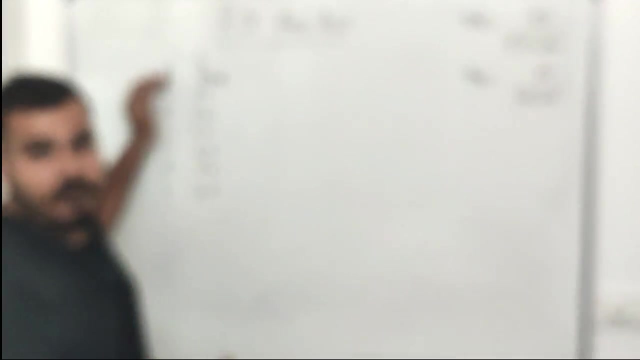 show that, how your model is actually performing in the form of some graphs, Then only the domain expert person will be able to help you out. So let us go and try to understand how to construct ROC and AUC curve, what exactly it is, and we'll just be discussing about this in this specific video, So make sure that you watch this video till the end. So let us take an example Here. I have an output value of my use case, which is Y, which is my actual value. So I have values like 1 0, 1, 1 0, 1.. 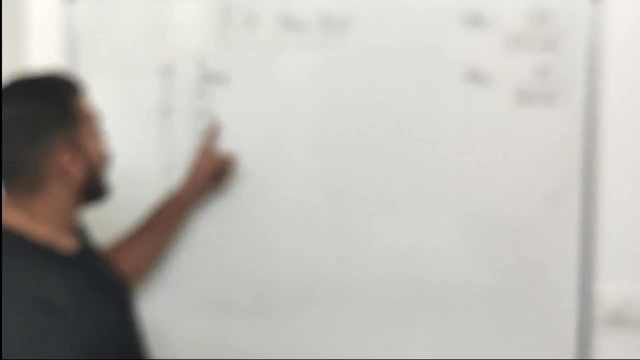 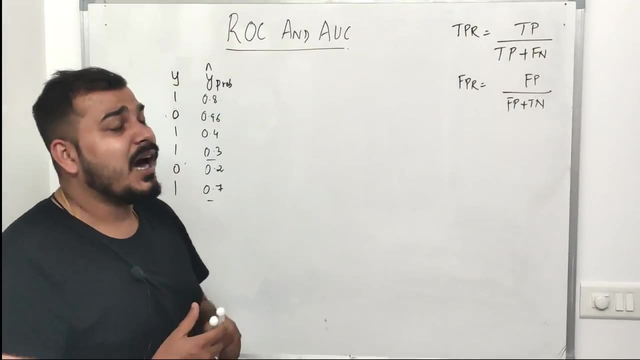 And my model is actually predicted a probabilities like 0.8, 0.96, 0.4, 0.3, 0.2, 0.7.. Suppose it has predicted like this. Now for constructing the ROC and AUC curve, we will be considering some threshold values. 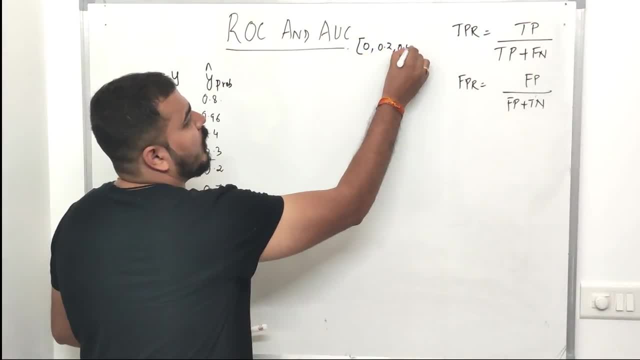 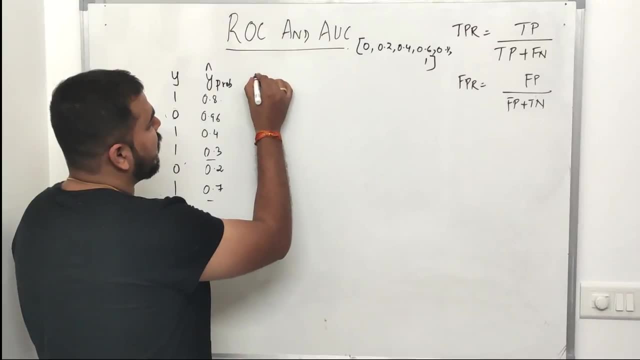 Okay, So suppose I start with 0, then 0.2, 0.4,, 0.6,, 0.8 and 1.. Right, These are my threshold values. Okay, So, first off, the thing is that I will try to suppose if I set up my threshold value. 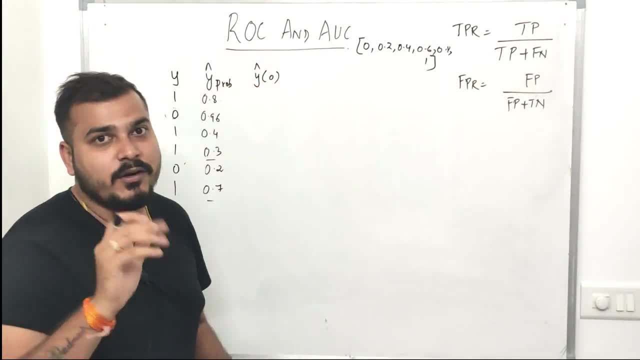 as 0, then what will be my Y hat? Okay, We will try to understand. So we know that 0.8 is greater than 0. So, definitely, if it is greater than the threshold value, it is going to become 1.. 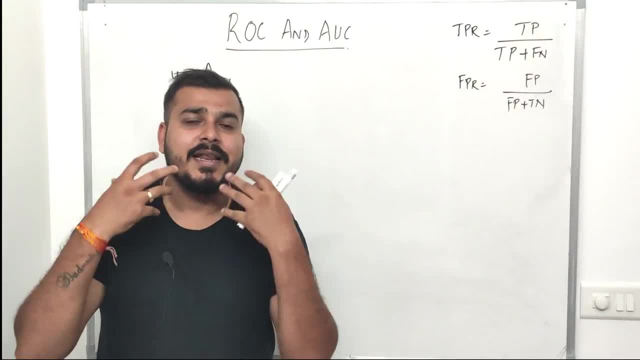 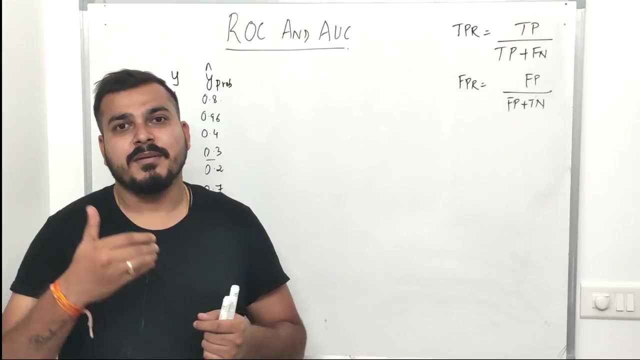 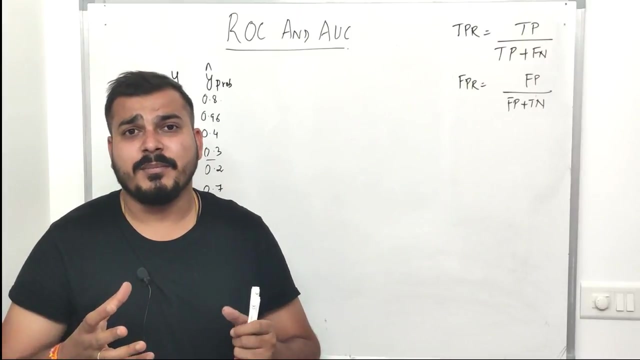 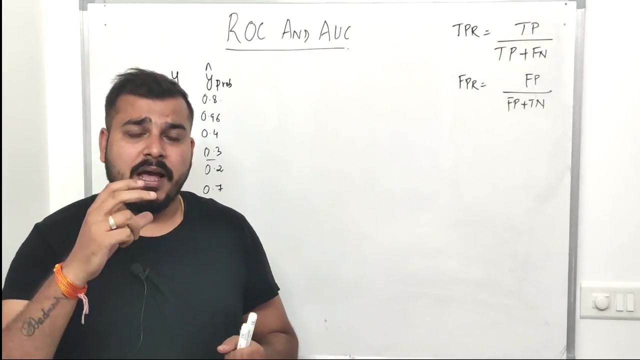 Now let me just take some examples about it. Suppose you are working in a healthcare domain project and the model that it is predicting it is very, very critical. You know it may be a disease patient, it may be something. So at that time you know what may happen- is that the threshold value that should be kept, based on the type of problem statement. Suppose you want higher true positive rate, you want less false positive rate. So based on that, we can actually play with the threshold and again, a domain expert person will always be there, will be able to guide you out. But remember, guys, you need to 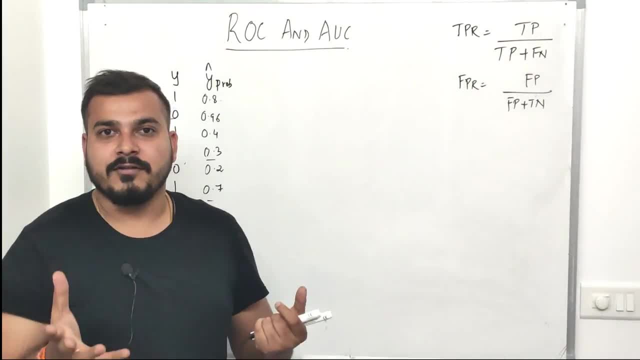 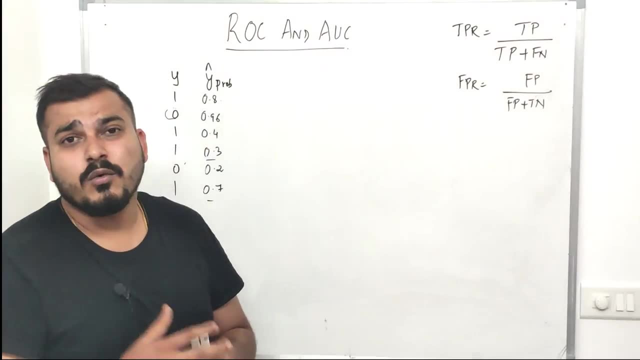 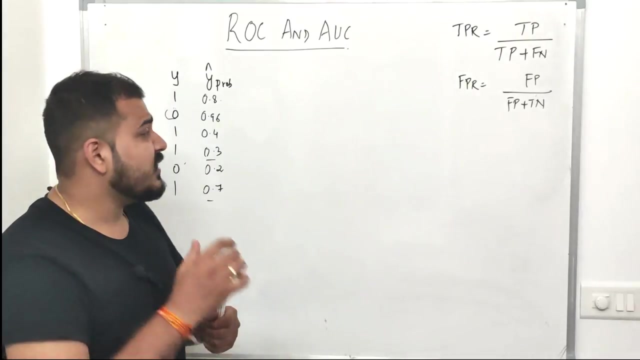 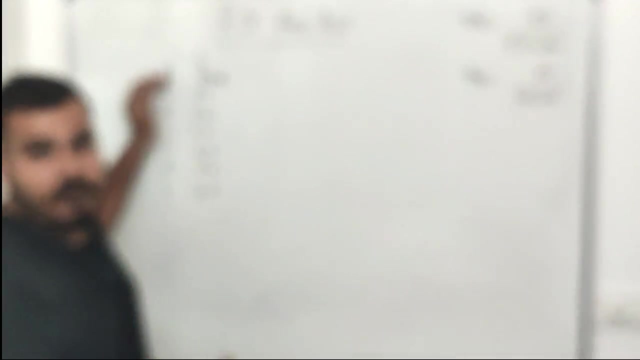 show that, how your model is actually performing in the form of some graphs, Then only the domain expert person will be able to help you out. So let us go and try to understand how to construct ROC and AUC curve, what exactly it is, and we'll just be discussing about this in this specific video, So make sure that you watch this video till the end. So let us take an example Here. I have an output value of my use case which is Y. Okay, which is my actual value. Okay, so I have values like 1 0 1 1 0, 1.. Okay, and I have an output value of my use case which is Y. Okay, so I have values like 1 0 1, 1 0, 1.. Okay, and I have an output value of my use case which is Y. Okay, so I have values like 1 0 1 1 0, 1.. Okay, and I have an output value of my use case which is Y. Okay, so I have values like 1 0 1 1 0, 1.. Okay, and I have an output value of my use case which is Y. Okay, so I have values like 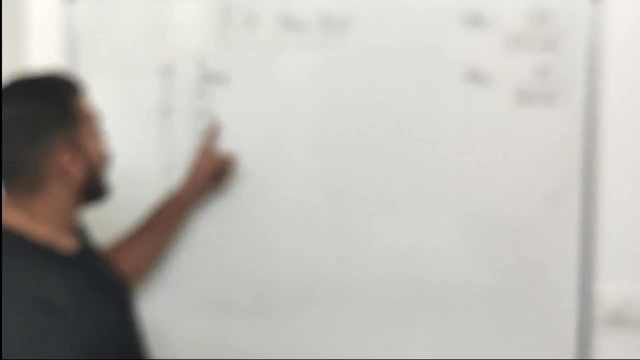 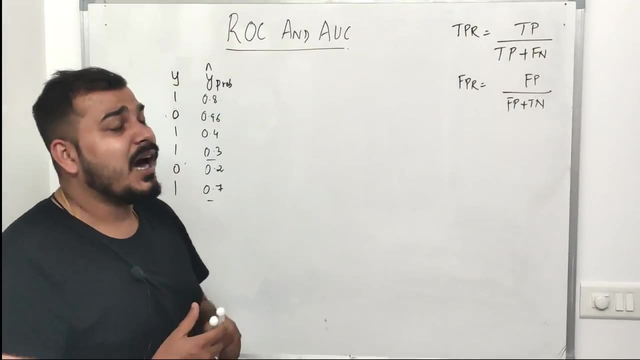 And my model is actually predicted a probabilities like 0.8, 0.96, 0.4, 0.3, 0.2, 0.7.. Suppose it has predicted like this. Now for constructing the ROC and AUC curve, we will be considering some threshold values. 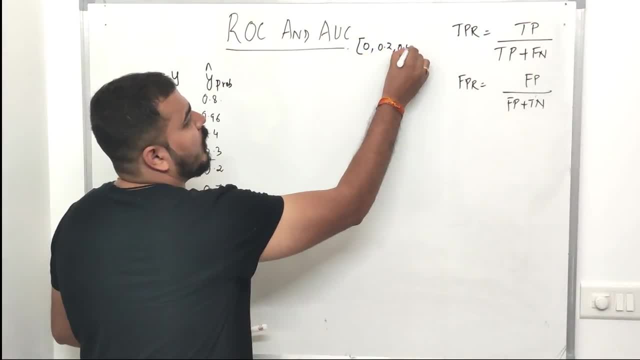 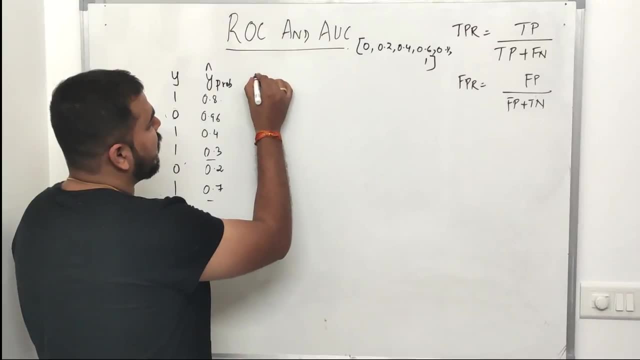 Okay, So suppose I start with 0, then 0.2, 0.4,, 0.6,, 0.8 and 1.. Right, These are my threshold values. Okay, So, first off, the thing is that I will try to suppose if I set up my threshold value. 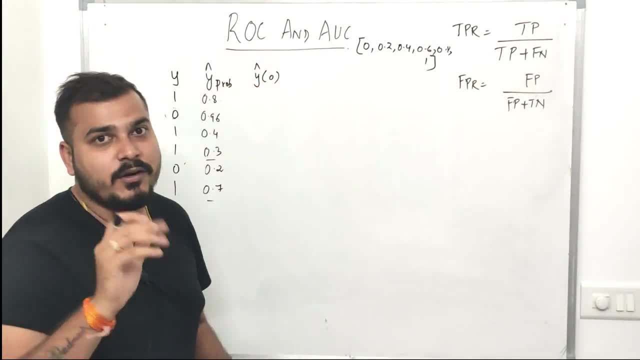 as 0, then what will be my Y hat? Okay, We will try to understand. So we know that 0.8 is greater than 0. So, definitely, if it is greater than the threshold value, it is going to become 1.. 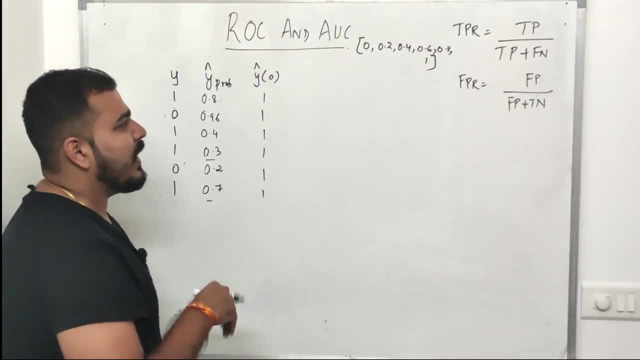 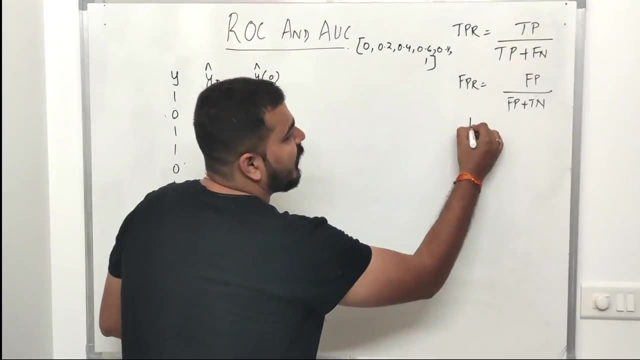 So all these values will actually become 1.. Now, once we have this right, we will try to capture, or we will try to calculate the true positive and the false positive rate. So suppose, if I want to calculate a true positive rate, it is nothing but TP divided by TP plus. 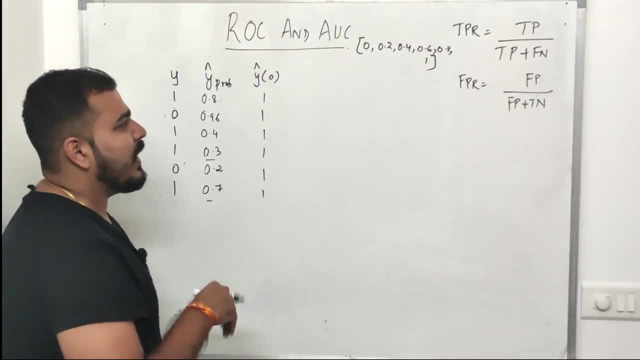 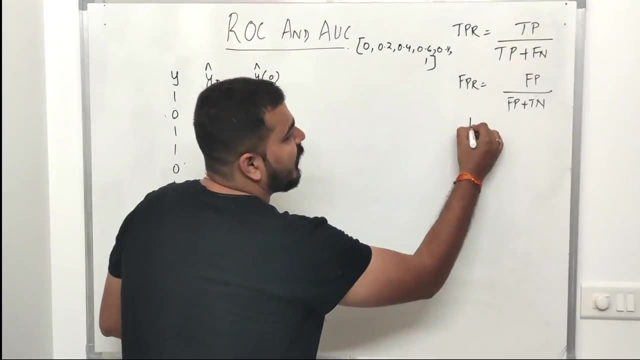 So all these values will actually become 1.. Now, once we have this right, we will try to capture, or we will try to calculate the true positive and the false positive rate. So suppose, if I want to calculate a true positive rate, it is nothing but TP divided by TP plus. 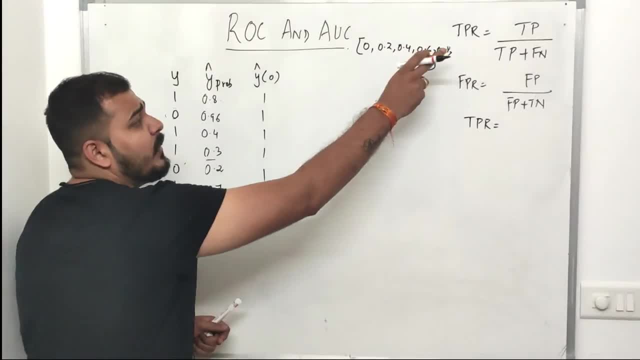 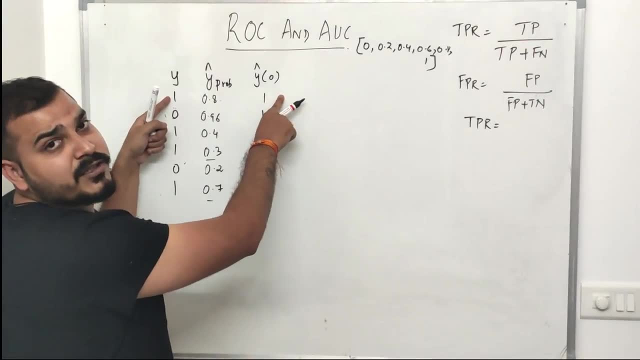 FN: Right, Pretty much simple. So here how many true positives I have. See What is true positives. Suppose my actual value is 1.. My output predicted value is 1.. These two are true positive. So I have 1 true positive, 2 true positive, 3 true positive and 4 true positives. 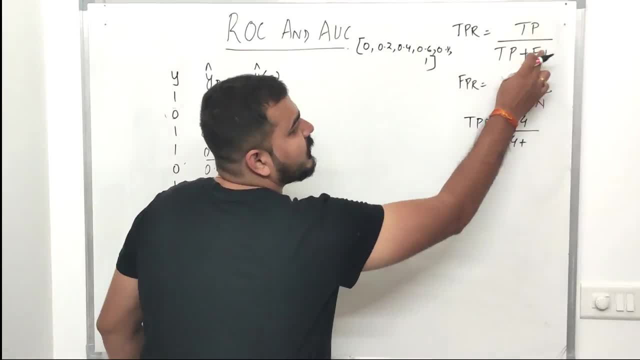 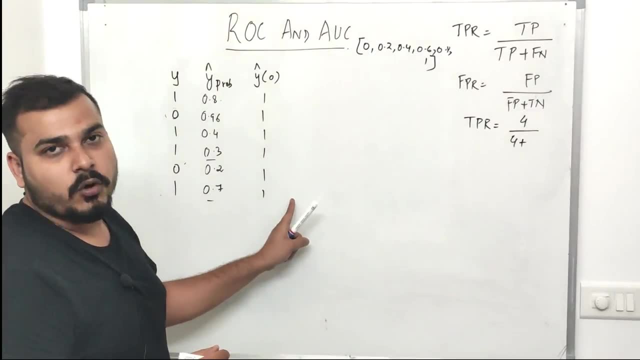 So total number of 4 true positives divided by 4 plus What is this FN? False negative basically means that suppose if I have 1 over here, my predicted value is 0.. Right, That is actually false negative In this scenario. I don't have those scenarios. 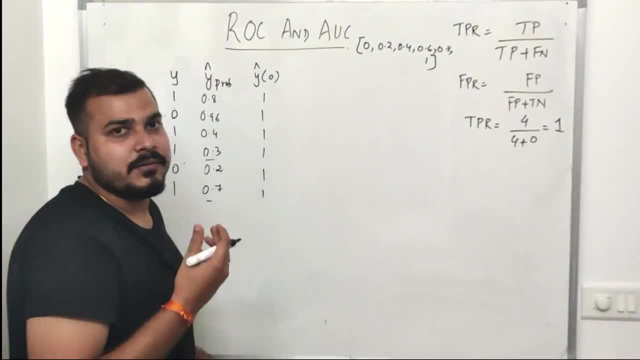 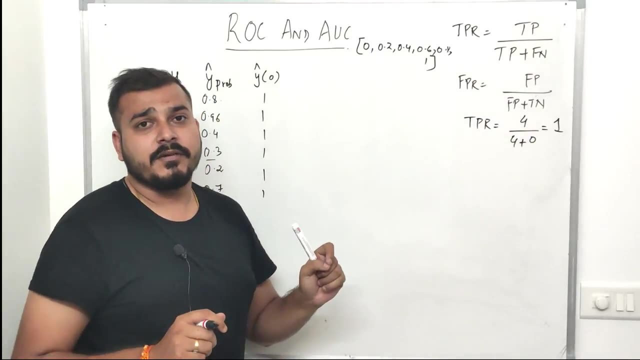 Right, So this will basically become 0.. Now I have 1 as my output. Fine, I got my true positive rate and remember, for ROC we require both true positive and false positive rate, because for the construction of graph we will be actually requiring it. 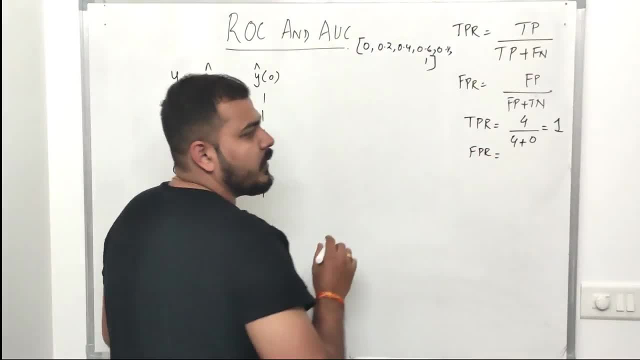 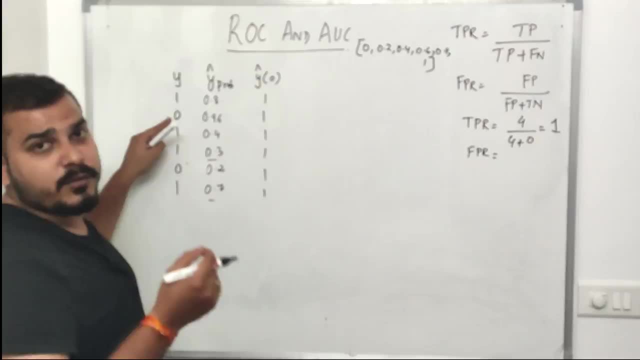 Now let us go ahead and calculate my false positive rate. Now, my false positive rate basically says false positive divided by false positive plus true negative. Now, in this particular scenario, what is false positive When my output value is 0, my predicted value is 1.. 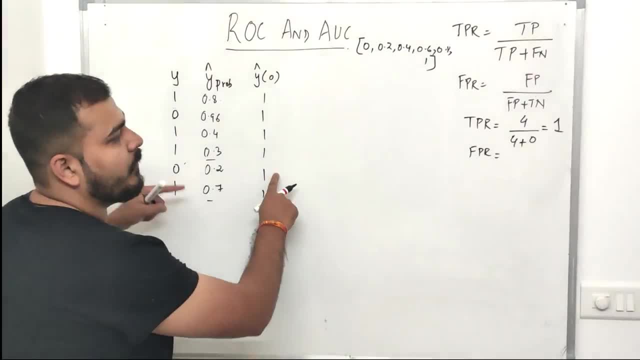 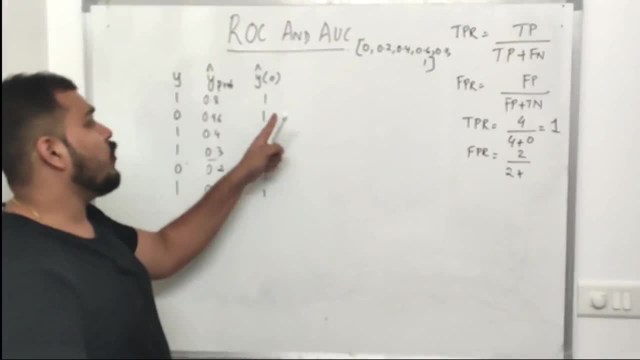 This is basically false positive. So I have 1 over here, 2 over here, So I am going to write it at 2.. 2 plus what about true negative? True negative basically means if your value is 0, the output value is also 0.. 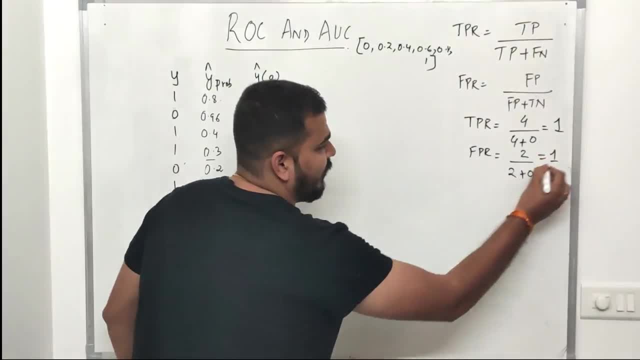 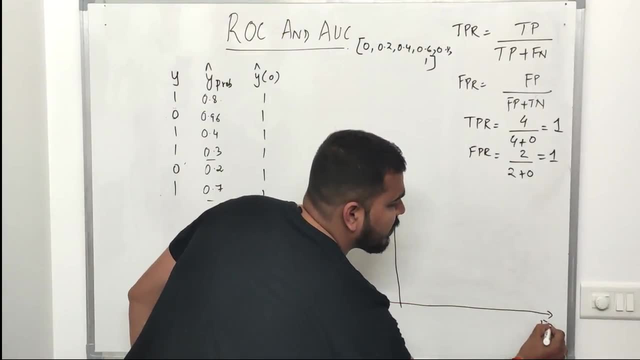 Right. So in this scenario it is 0.. So my total value is 1.. Now understand one thing. I am going to construct a graph. in the right hand side, In the x-axis, I have false positive rate. Over here I have true positive rate. 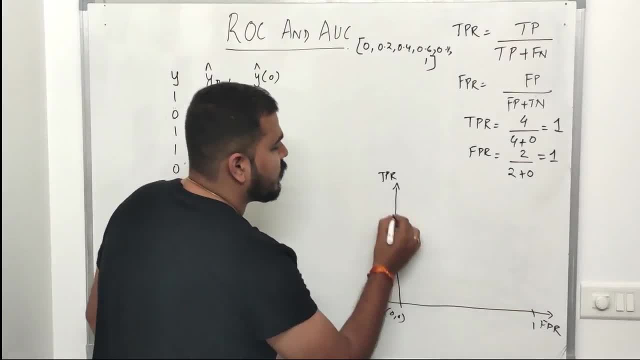 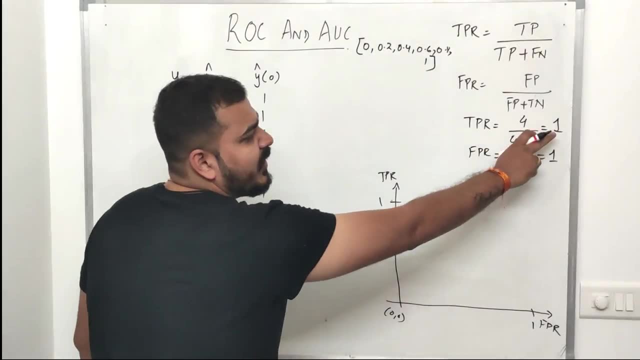 This is my 0, 0.. Remember my false positive rate? This is 1.. This is 1.. Right Now, you can understand that when my threshold was 0. I got my true positive rate as one, false positive rate, as one for this specific model. 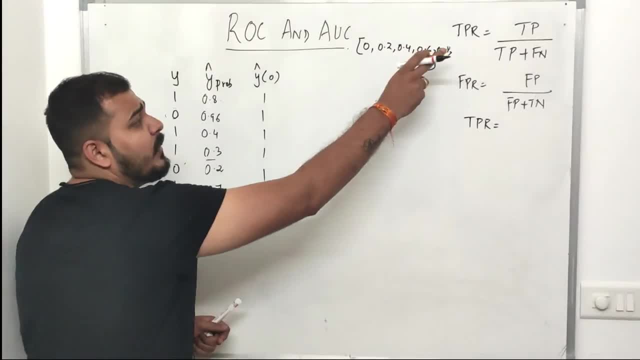 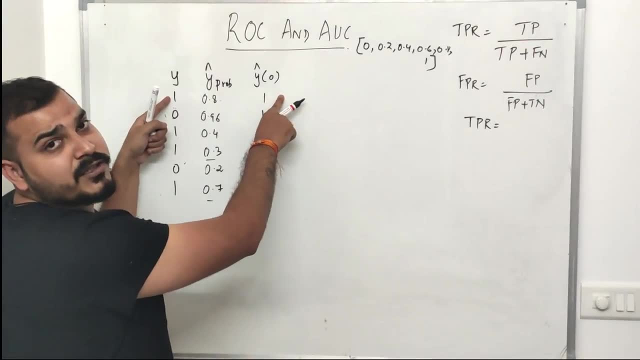 FN: Right, Pretty much simple. So here how many true positives I have. See What is true positives. Suppose my actual value is 1.. My output predicted value is 1.. These two are true positive. So I have 1 true positive, 2 true positive, 3 true positive and 4 true positives. 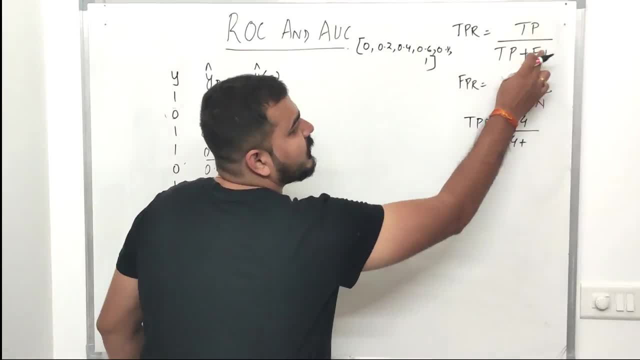 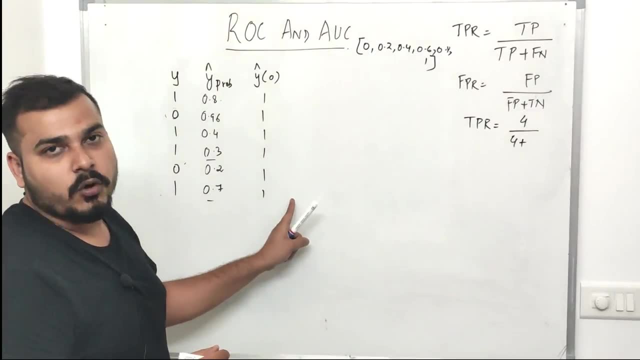 So total number of 4 true positives divided by 4 plus What is this FN? False negative basically means that suppose if I have 1 over here, my predicted value is 0.. Right, That is actually false negative In this scenario. I don't have those scenarios. 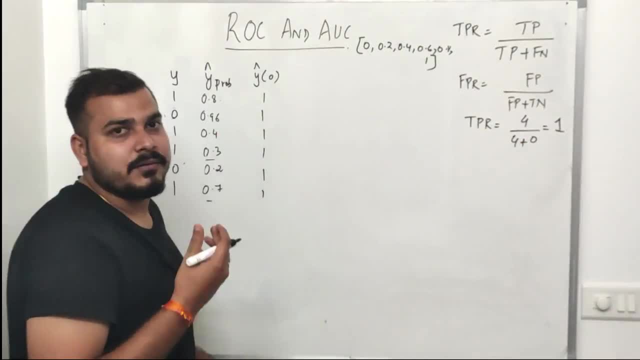 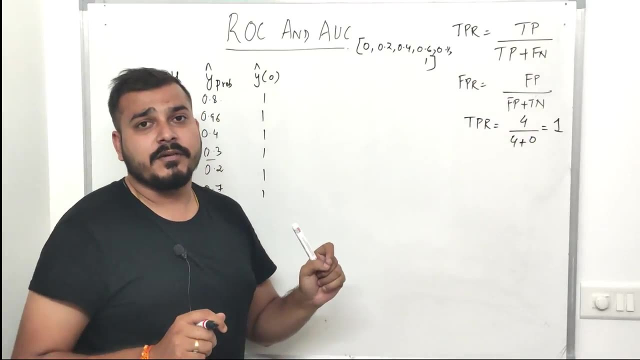 Right, So this will basically become 0.. Now I have 1 as my output. Fine, I got my true positive rate and remember, for ROC we require both true positive and false positive rate, because for the construction of graph we will be actually requiring it. 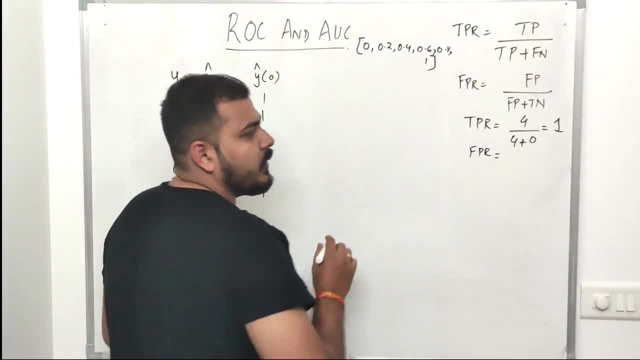 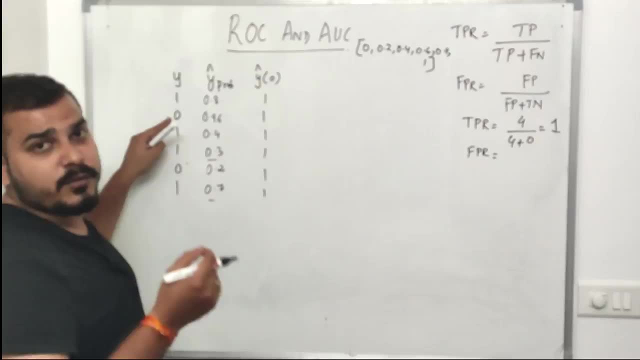 Now let us go ahead and calculate my false positive rate. Now, my false positive rate basically says false positive divided by false positive plus true negative. Now, in this particular scenario, what is false positive When my output value is 0, my predicted value is 1.. 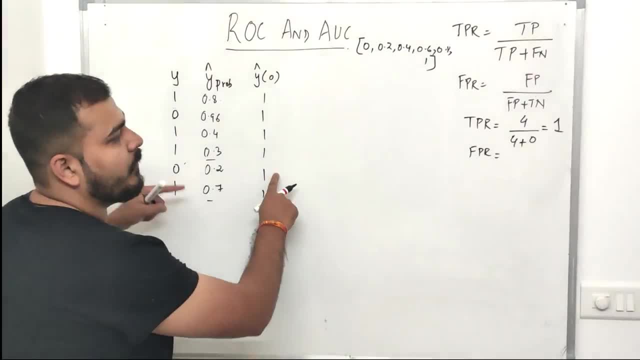 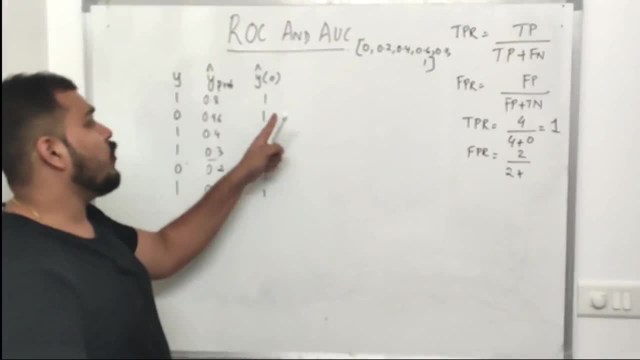 This is basically false positive. So I have 1 over here, 2 over here, So I am going to write it at 2.. If I write it at 2 plus, what about true negative? True negative basically means if your value is 0, the output value is also 0.. 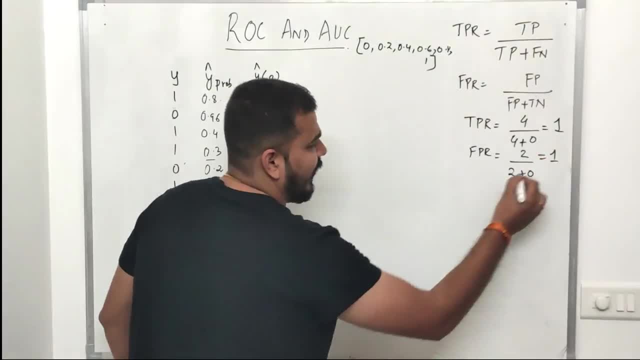 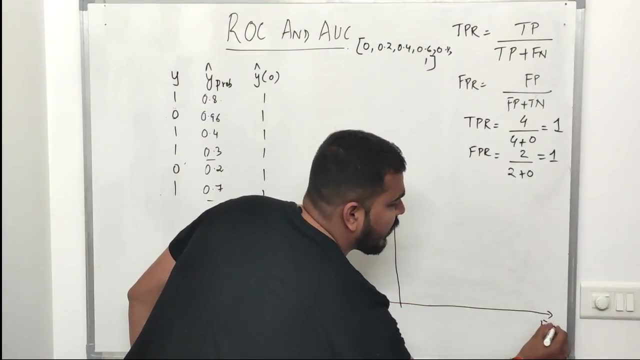 Right. So in this scenario it is 0.. So my total value is 1.. Now understand one thing. I am going to construct a graph. in the right hand side, In the x-axis, I have false positive rate. Over here I have true positive rate. 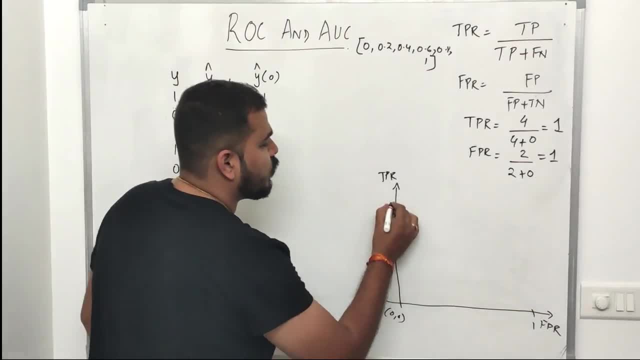 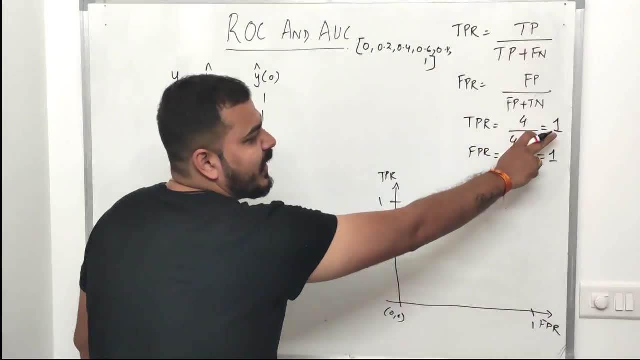 This is my 0, 0.. Remember my false positive rate? This is 1.. This is 1.. Right Now, you can understand that when my threshold was 0. I got my true positive rate as 1, false positive rate as 1 for this specific model. 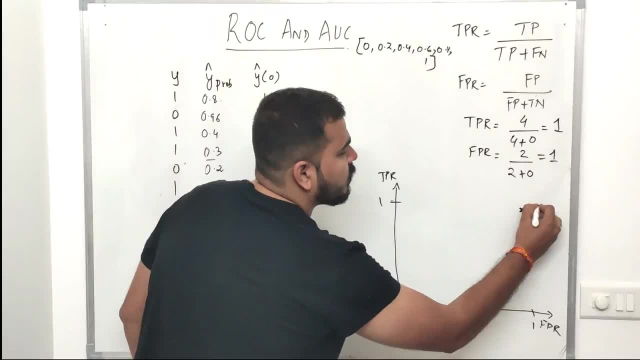 So if I go and try to point it out, it will come somewhere here. So this is basically 1, 1.. Right, My false positive rate is 1.. My true positive rate is 1.. When my threshold value is 0.. 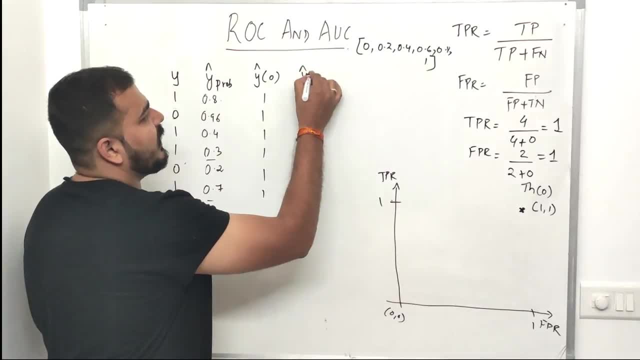 Right, Note it down. Now the next thing. Let me take the next value: y hat is 0.2.. Right, So anything greater than 0.2 is going to become 1.. In this case, this will become 1.. 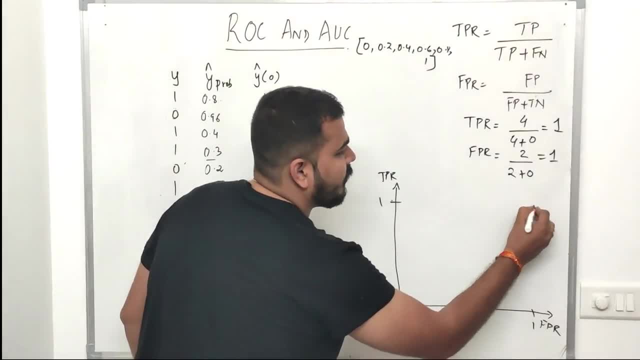 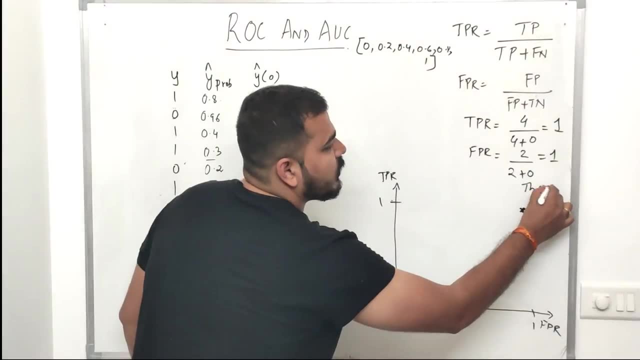 So if I go and try to point it out, it will come somewhere here. So this is basically 1 comma 1, right. My false positive rate is 1. my true positive rate is 1 when my threshold value is 0. Right, noted down. now the next thing. Let me take the next value: y hat is 0.2. 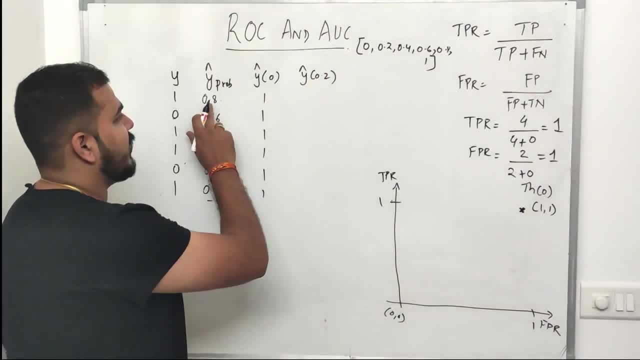 Right. So anything greater than 0.2 is going to become 1. in this case, This will become 1. this will become 1. 1, 1. This will be 0. this will be 1, because here I have 0.2 only. 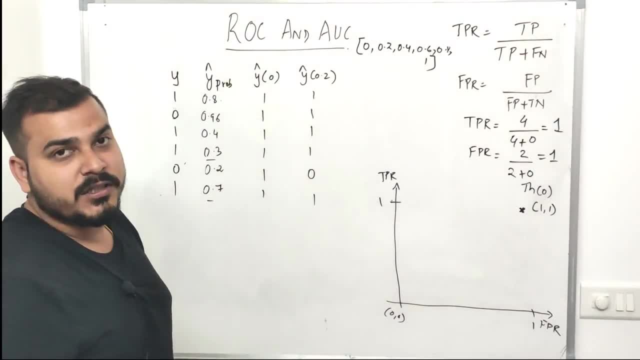 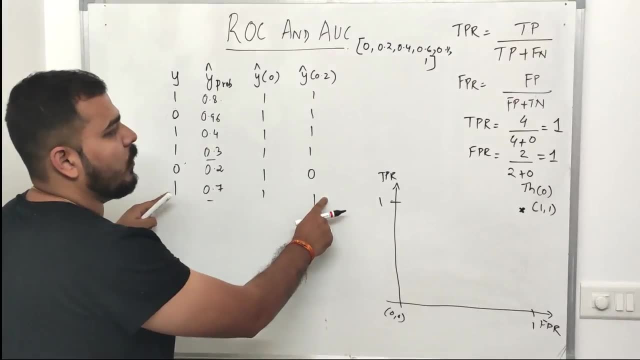 Okay, Now if I go and calculate, calculate the true positive rate, what it will be again How many true positive rate. over here I have 1. over here I have 1. 1, 2, 3, 4. so my true positive rate will be 1 only. 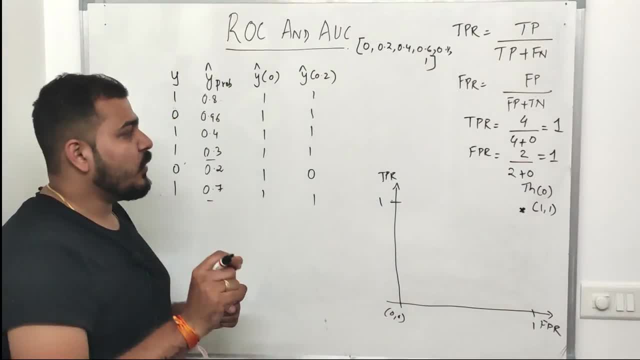 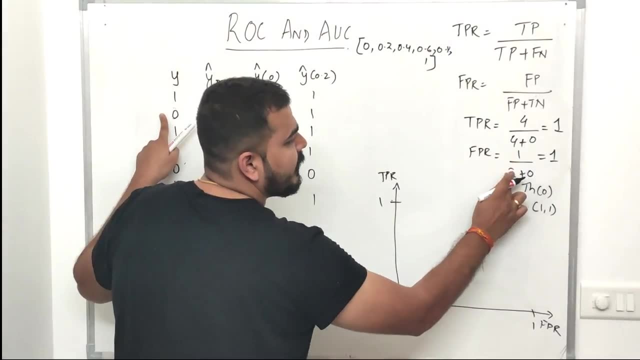 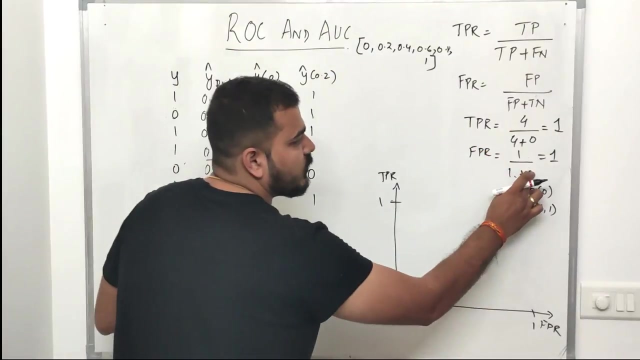 Okay, what about my false positive rate? now try to understand how many false positive are there? only one false positive, are there, Right? So my false positive rate will become 1 divided by 1 plus. what about my true Negative? now you can see there is a one true negative, right? So this will become 1. 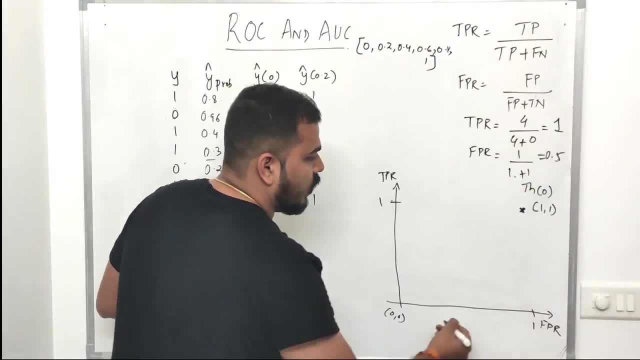 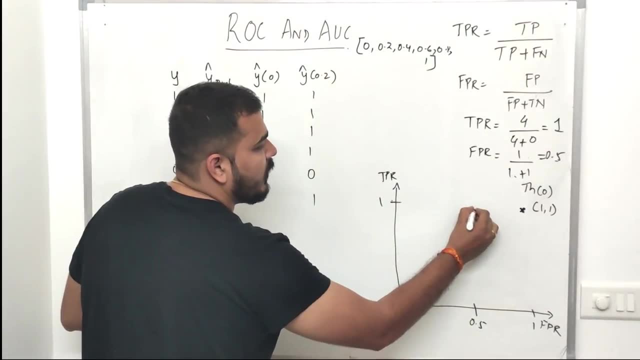 So 1 divided by 2 is nothing but 0.5. So my false positive rate is 0.5 over here. My true positive rate is somewhere over here. So I'm going to get this value and I am going to rate it as 0.5 comma 1 for my threshold value. 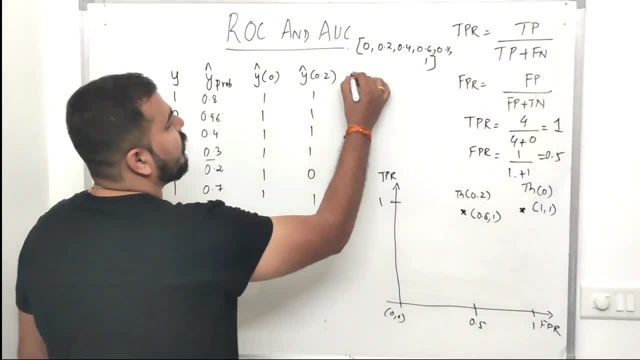 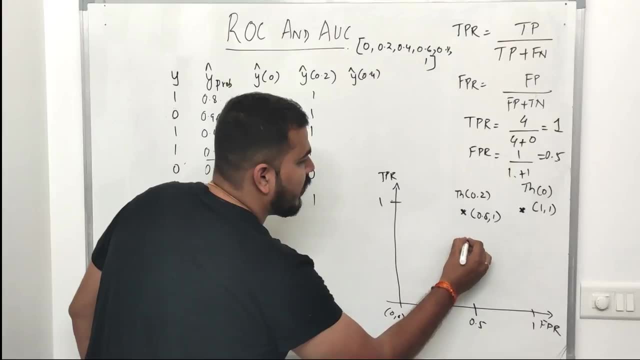 0.2 Right Now. similarly, when we start doing these things for all the values, We will be getting some kind of graph. suppose My third point will be somewhere here, and this will be somewhere like 0.5 comma 0.6 for threshold of 0.4. 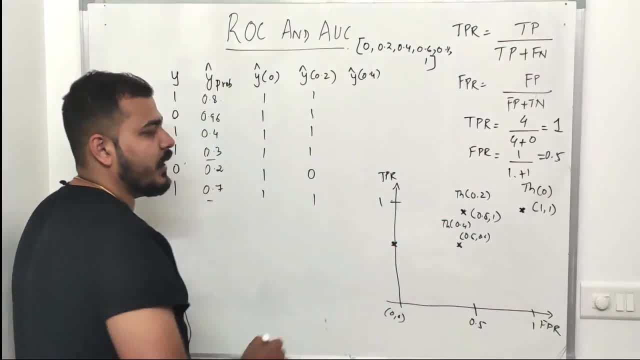 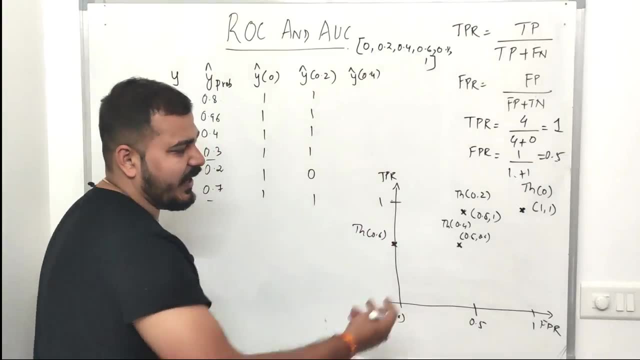 Okay, we'll be constructing this graph. Okay, then one more point will be coming over here, right? So here, basically, my false positive. again, this will be my for my threshold: 0.6, I guess 0.8. so this kind of graph will get created and finally, one point will be here. 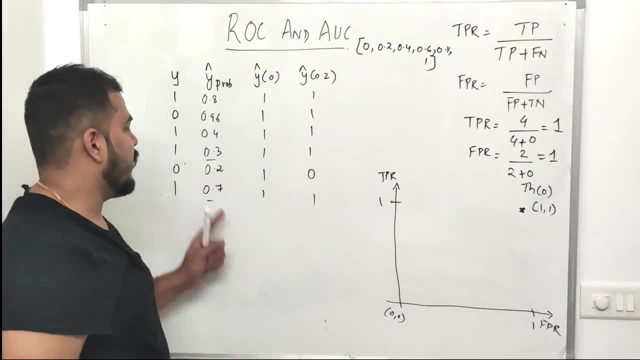 This will become 1, 1, 1. This will be 0. This will be 1. Because here I have 0.2 only. Okay, Now, if I go and calculate the true positive rate, What it will be. 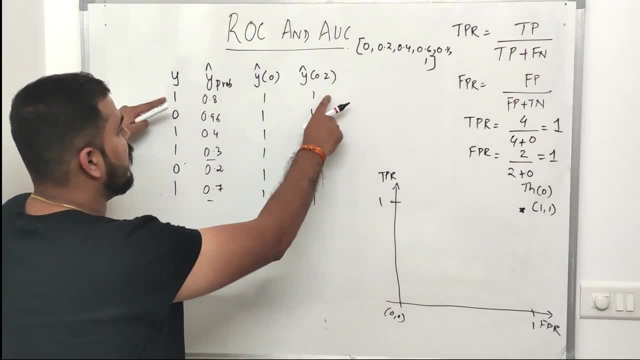 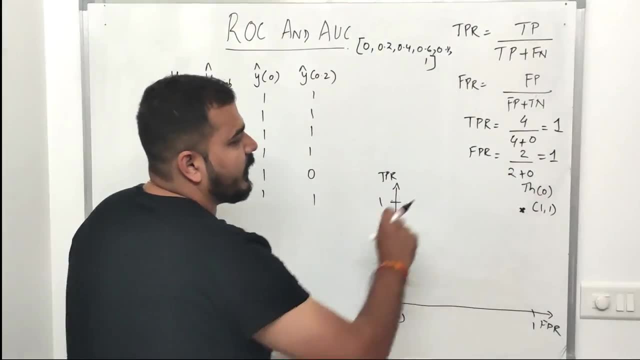 Again, How many true positive rate Over here I have: 1. Over here I have 1.. 1,, 2,, 3,, 4.. So my true positive rate will be 1 only. Okay, What about my false positive rate? 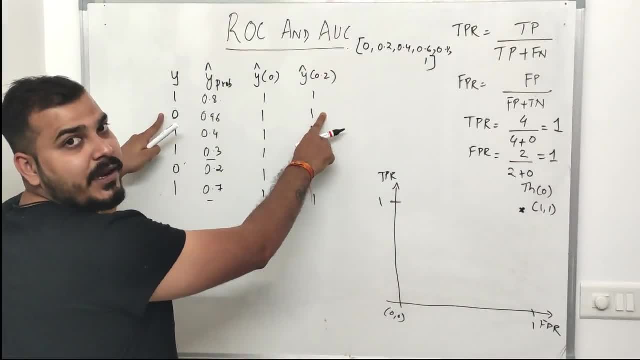 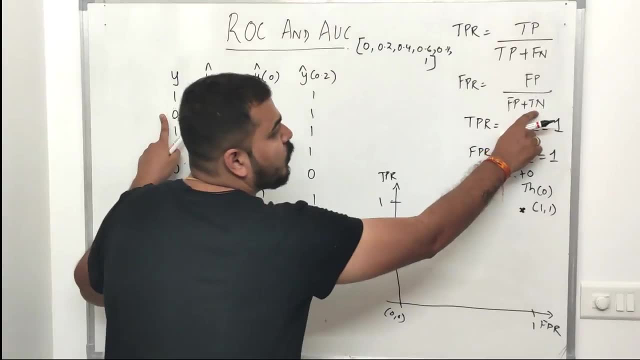 Now try to understand. how many false positive are there? Only 1 false positive are there, Right? So my false positive rate will become 1 divided by 1 plus What about my true negative? Now you can see there is a 1 true negative. 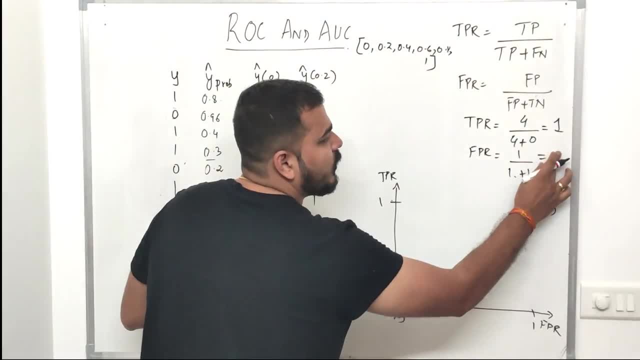 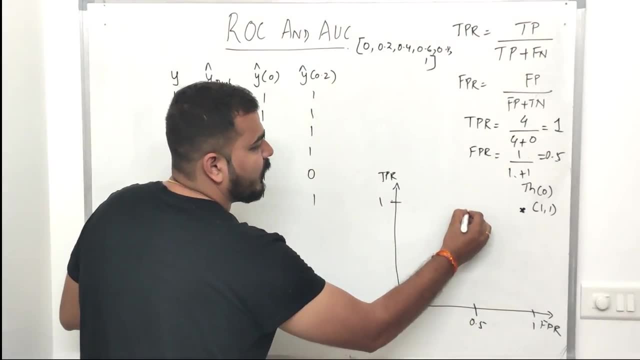 Right, So this will become 1.. So 1 divided by 2 is nothing but 0.5.. So my false positive rate is 0.5 over here. My true positive rate is somewhere over here. So I am going to get this value. 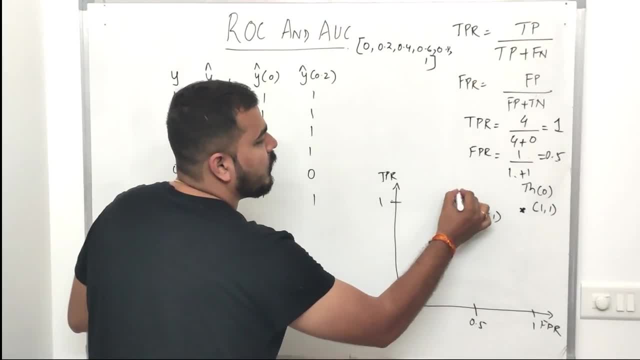 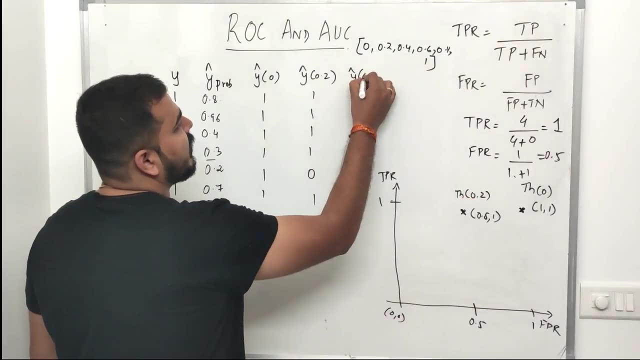 And I am going to rate it as 0.5 comma 1 for my threshold value 0.2.. Right Now, similarly, when we start doing these things for all the values, we will be getting some kind of graph, Suppose. my third point will be somewhere here. 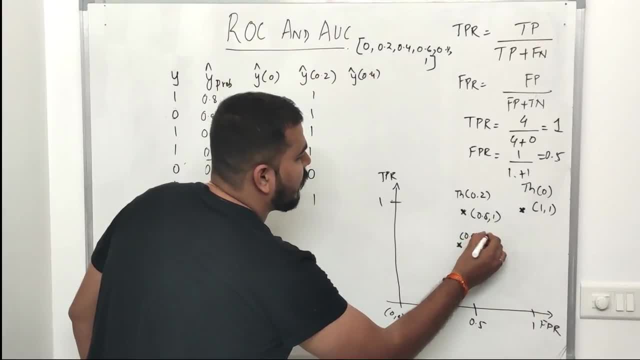 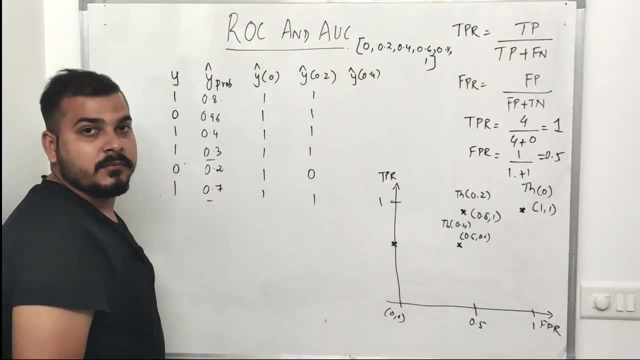 And this will be somewhere like 0.5 comma 0.6 for threshold of 0.4.. Okay, We will be constructing this graph. Okay, Then one more point will be coming over here, Right? So here, basically, my false positive. again, this will be for my threshold 0.6, I guess. 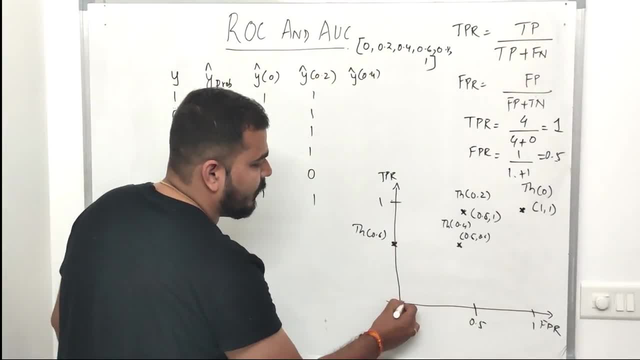 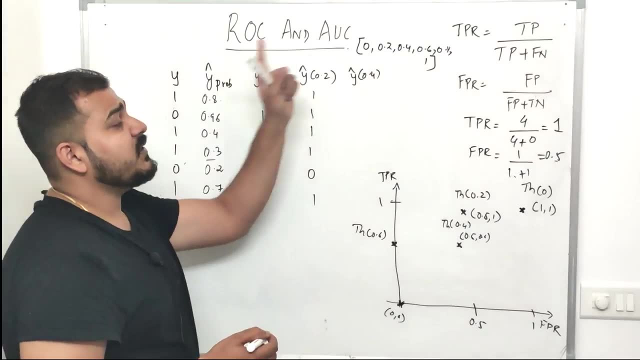 or 0.8.. So this kind of graph will get created And finally, one point will be here. Right Now, this whole thing is basically a ROC curve. Okay, Now you need to understand what is this AUC. 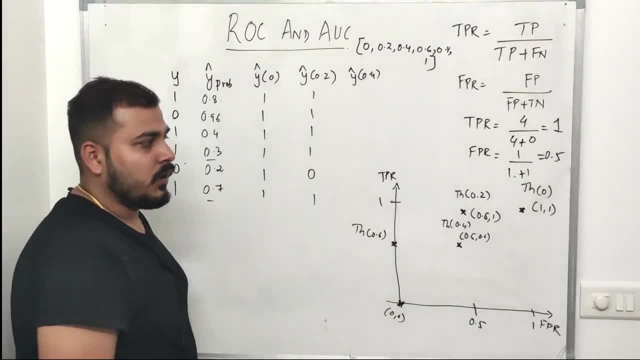 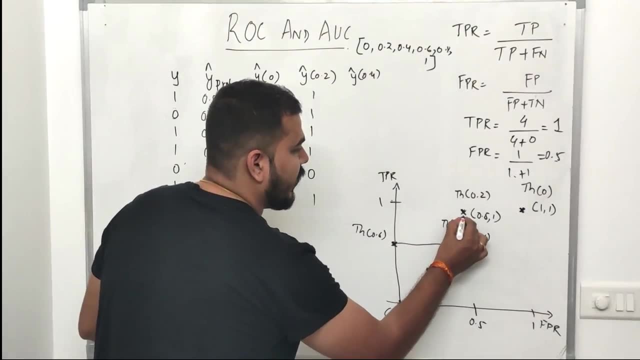 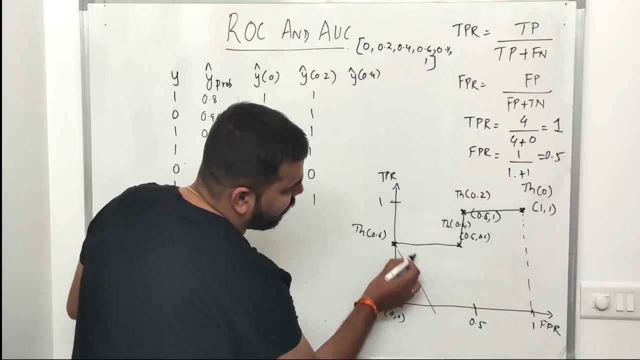 Right Now, this whole thing is basically a ROC curve. Okay, Now you need to understand what is this AUC? Now, when I connect all these points, all these dots together, all these dots together, So when I, when I, when I connect all these things, the curve that comes inside, this is basically my. 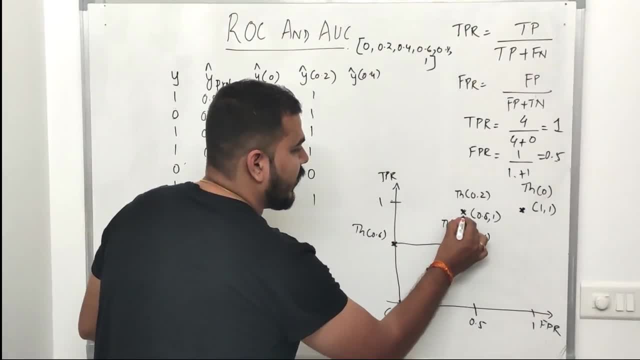 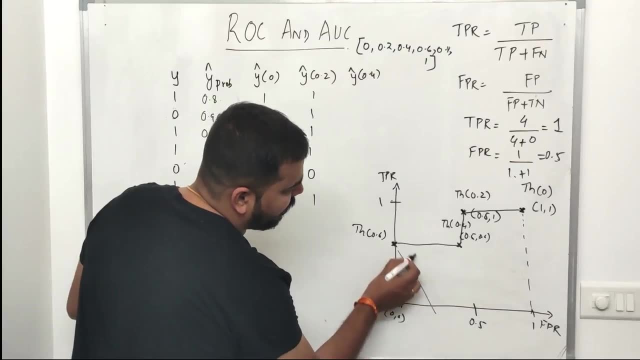 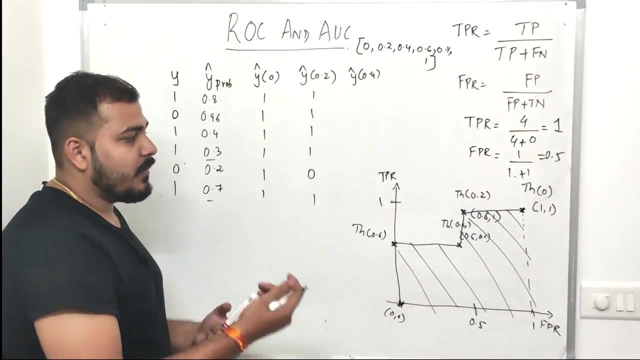 Now, when I connect all these points, all these dots together, all these dots together, So when I connect all these things, the curve that comes inside, this is basically my AUC curve area under the curve. And remember guys, the more the area under the curve, the better the model is yours. 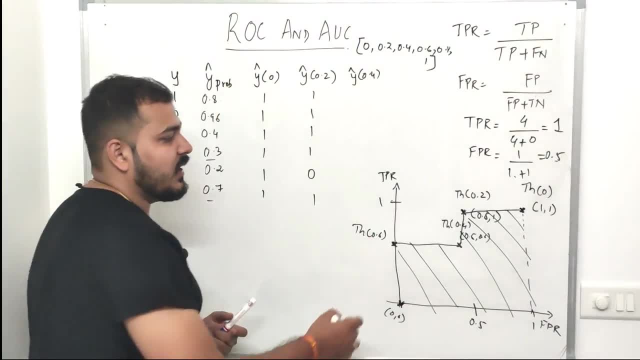 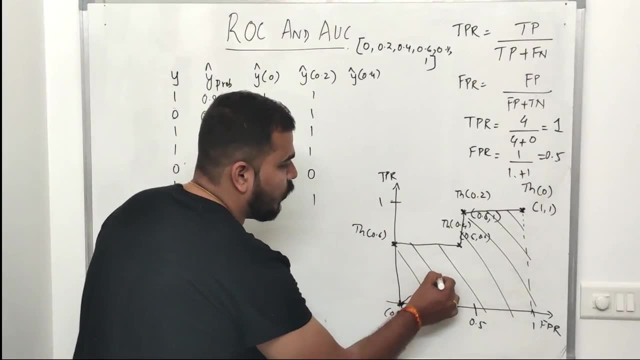 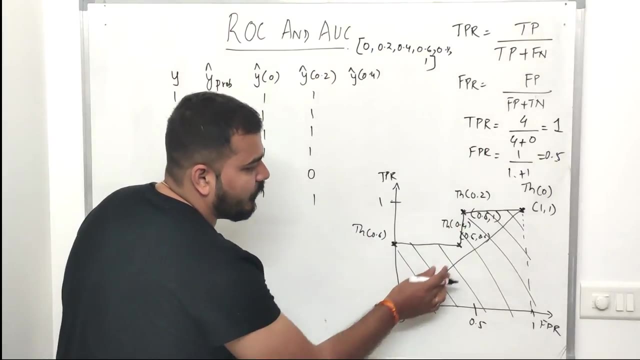 AUC curve area under the curve. and remember, guys, The more the area under the curve, the better the model is yours, right? So instead of this will, let me just also draw one line from the center. Okay, And always remember, a good model Should always be greater than this particular area. 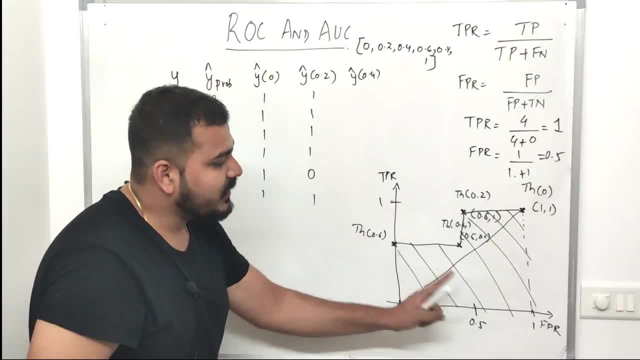 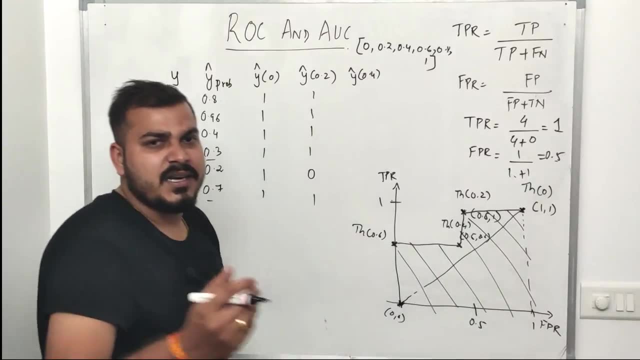 Greater than this particular area. It should never be less than this 0.5. Okay, this particular line that you see. right, it should always be greater than this, because if it is less than this, It is basically a dumb model, a model which is just random guessing right. 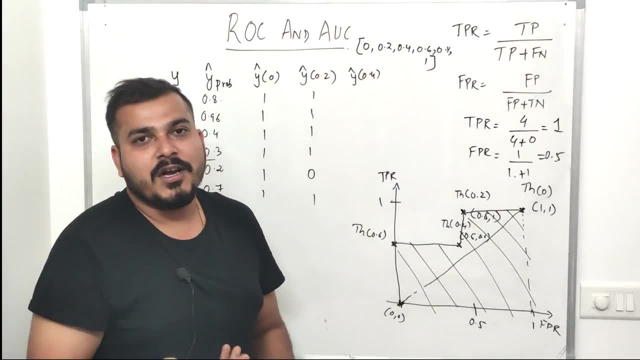 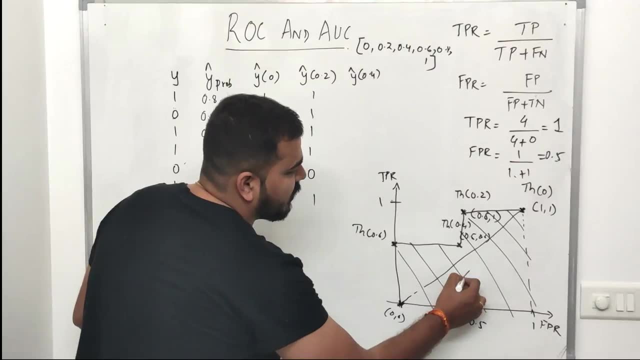 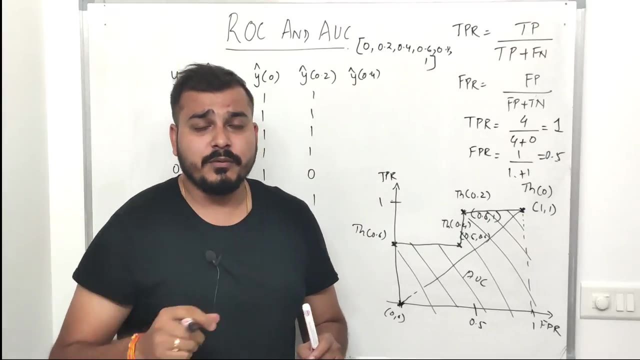 And if the probability is less than 0.5, I can just write a if cost and write that. sometime I can say it as 1, sometime I can say it as 0. So this is basically my AUC area under the curve now. Still, we did not decide what threshold value needs to be sure, needs to be selected from this particular use case. 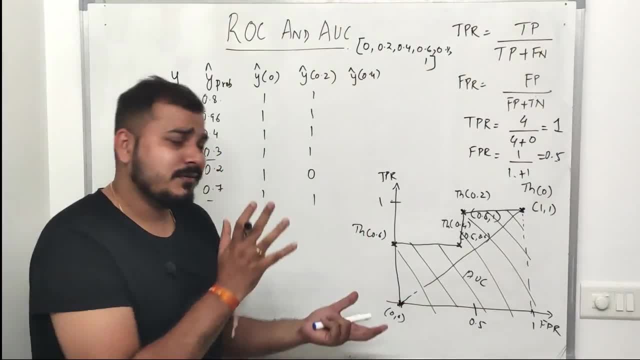 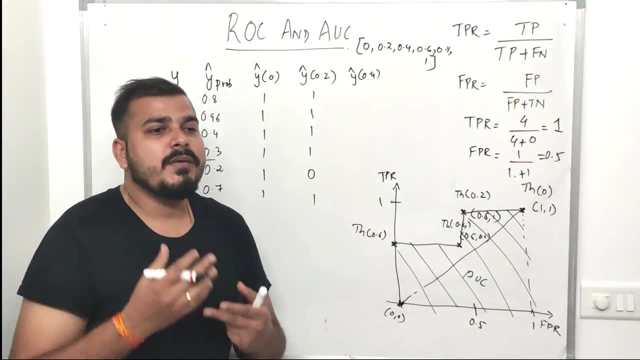 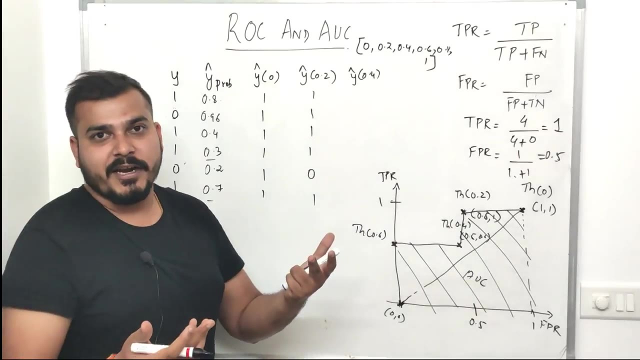 Now understand one thing, guys: if I take this problem statement, If I go and take this particular graph and show it to a domain expertise, The domain expertise will focus on saying that, Krish, we will be requiring higher true positive rate. now suppose, if I want to, You know, get more true positive rate or more true positive from this, I can select two values. one is this particular value. 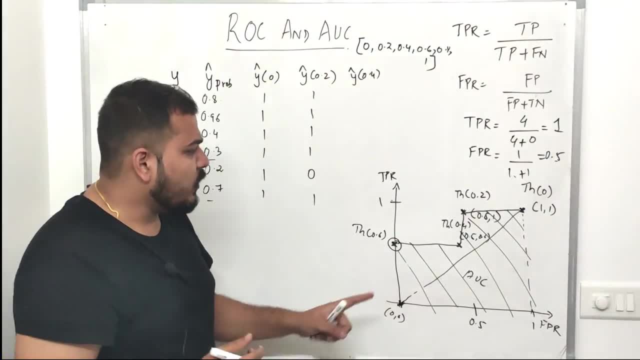 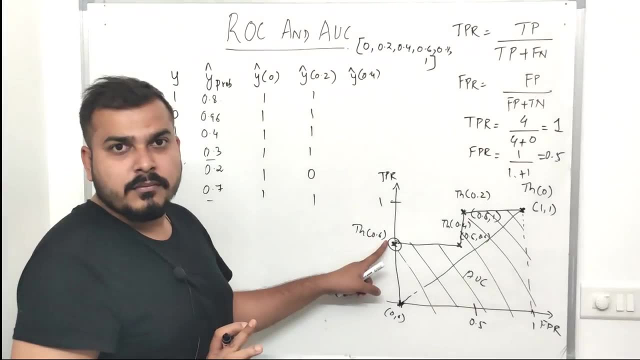 if he says that Krish only focus on true positive, then I can go and select this particular threshold, the threshold of 0.6, because in this scenario you can see that my fpr is 0, My false positive rate is completely zero. right, But suppose he says that Krish, come on. 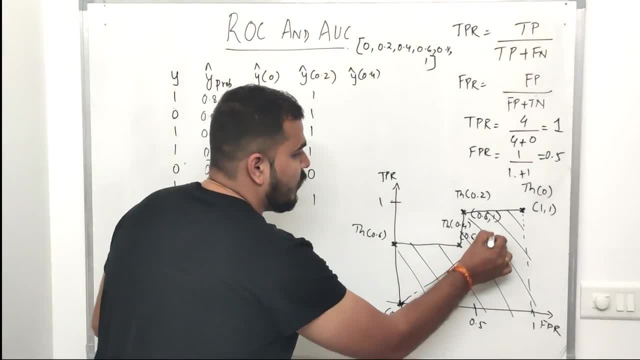 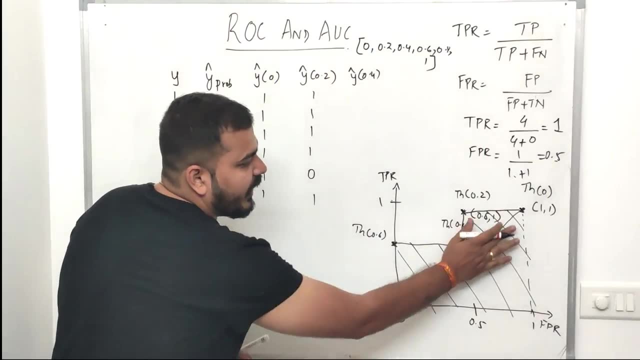 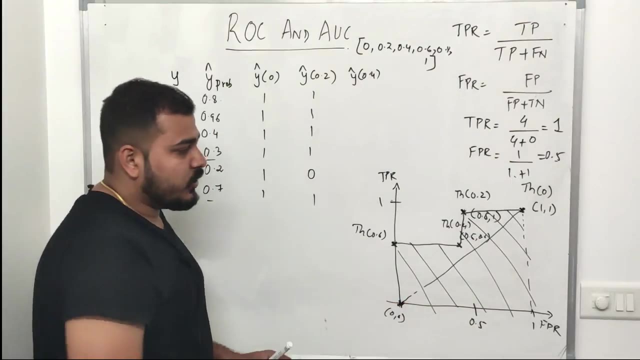 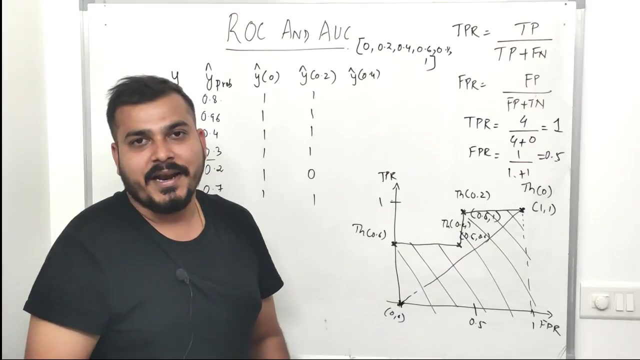 Right. So instead of this, let me just also draw one line from the center. Okay, And always remember, a good model should always be greater than this particular line, This particular area, greater than this particular area. it should never be less than this point five. okay, this particular line that you see. right, it should always be greater than this, because if it is less than this, it is basically a dumb model, a model which is just random, guessing right. and if the probability is less than point five, I can just write a if cost and write that. sometime I can say it as one, sometimes I can say it as zero. 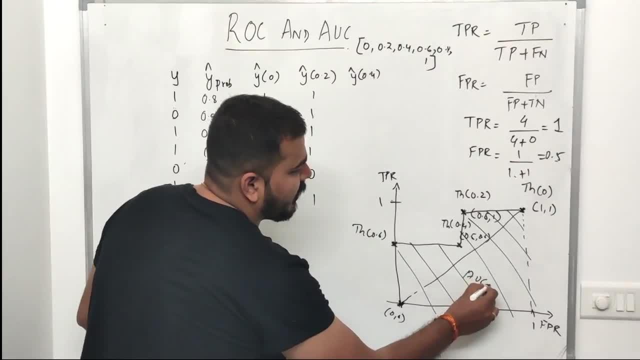 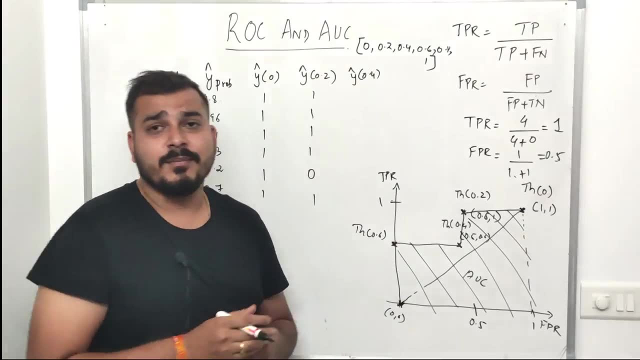 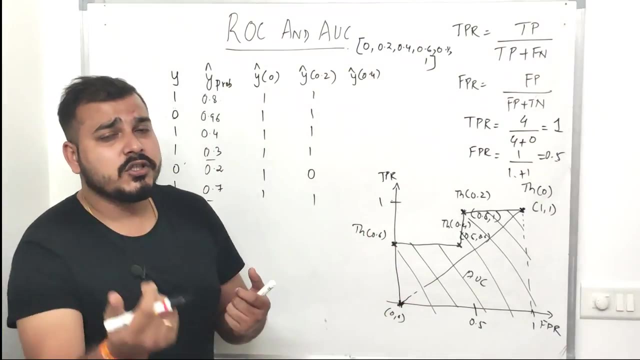 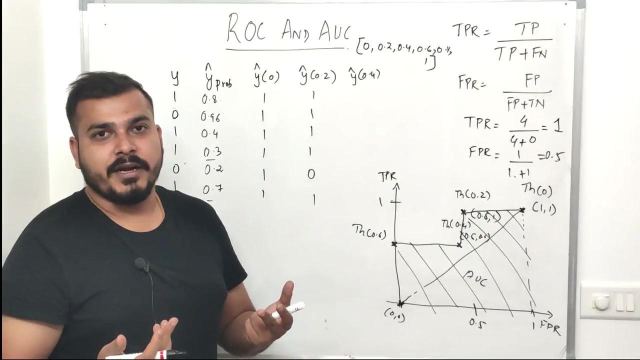 So this is basically my AUC area under the curve. Now, still, we did not decide what threshold value needs to be sure, needs to be selected from this particular use case. Now understand one thing, guys: if I take this problem statement, if I go and take this particular graph and show it to a domain expert, the domain expert will focus on saying that, Krish, we will be requiring higher true positive rate. 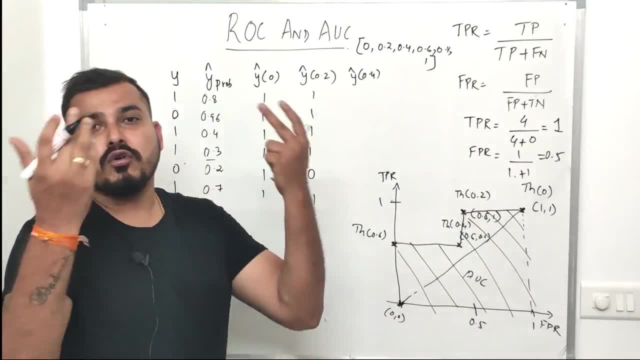 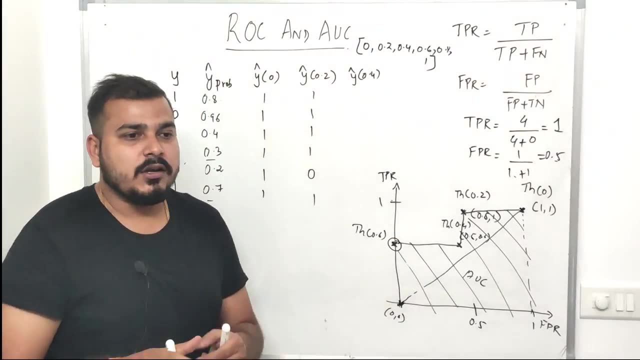 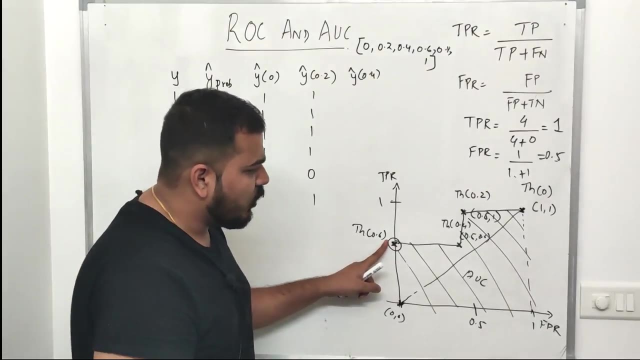 Now suppose, if I want to, you know, get more true positive rate or more true positive from this, I can select two values. one is this particular value. If he says that Krish only focus on true positive, Then I can go and select this particular threshold, the threshold of 0.6, because in this scenario, you can see that my FPR is zero, my false positive rate is completely zero, right? 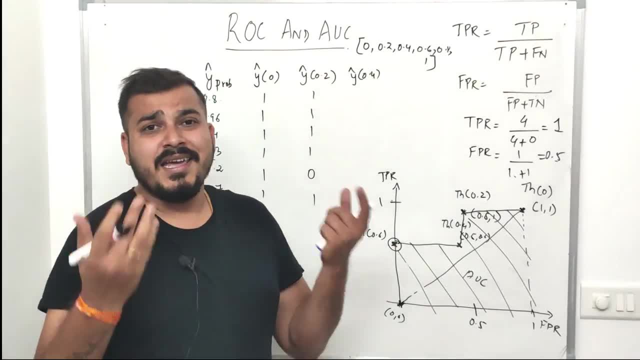 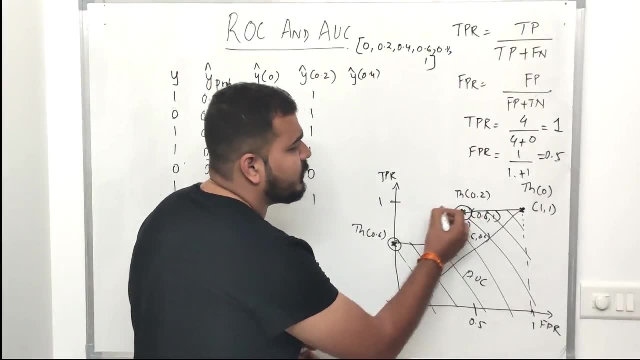 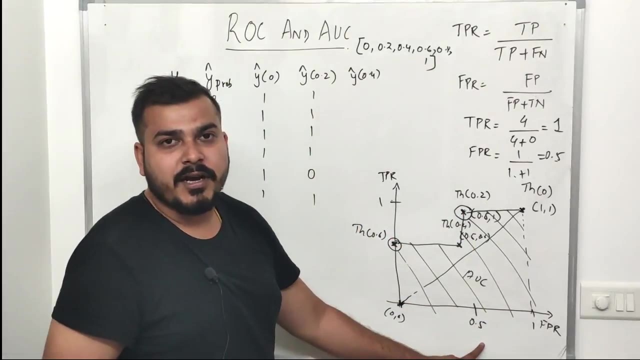 But suppose he says that, Krish, come on, I want high, more higher than this two positive rate. Okay, but I don't care about false positive. then what will happen is that I'll go and select this particular value. In this particular value, I'm getting one, two positive rate, but there is some amount of false positive rate. 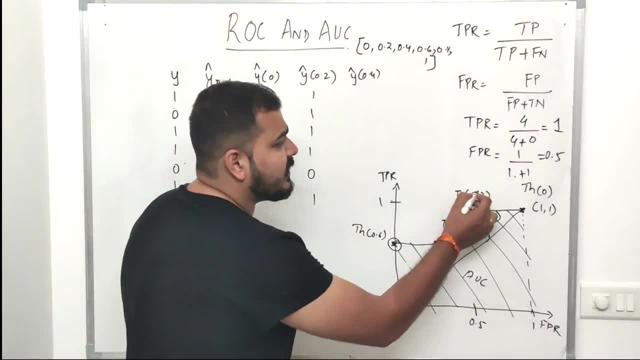 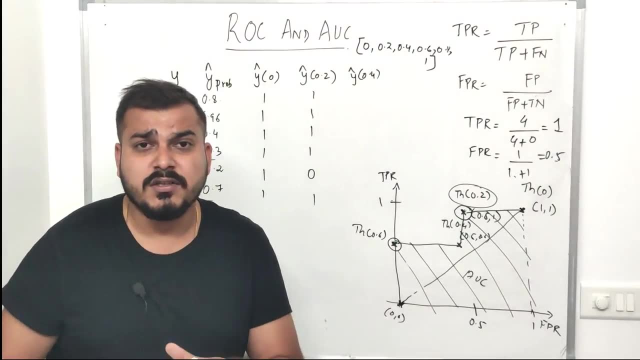 But he's saying that I do not care about that right. So at that time I can select this threshold values point to Right. Now suppose he says that, Chris, I- I mean I need to focus on both true positive and false positive. I need to see that particular result. I can also select this one. 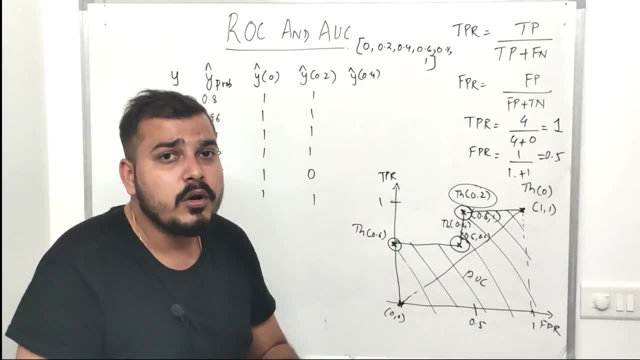 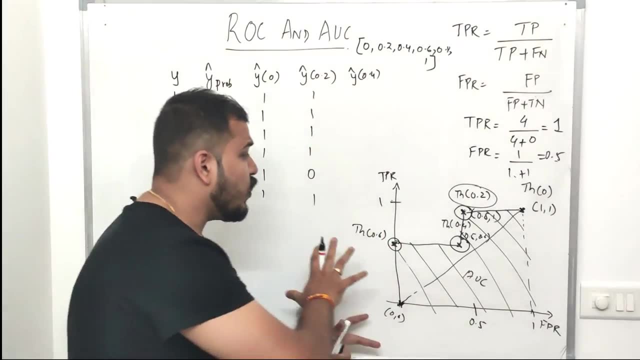 So it depends on the domain expert, a person, what they are looking at, how your model is actually performing and what is the data that you have represented in front of him. and Remember, guys, if you are able to explain him in this particular way, If you are able to show this particular diagram to him, then he'll be able to say: okay. 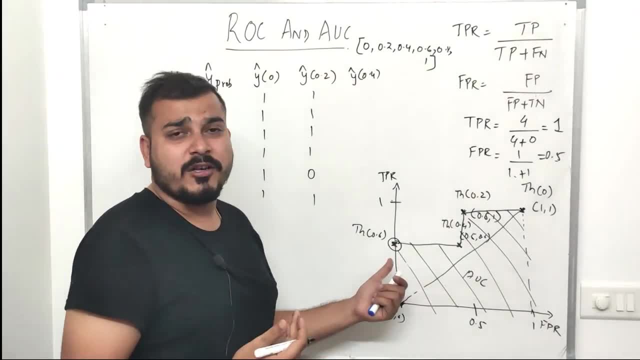 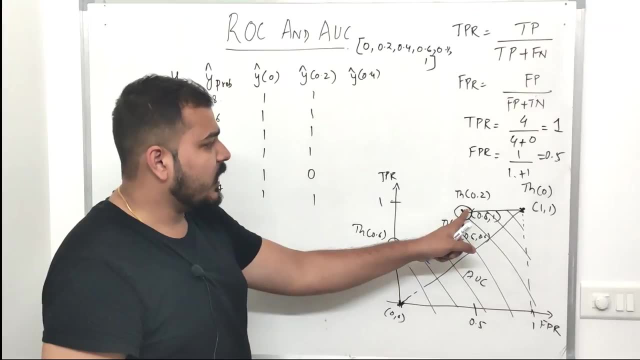 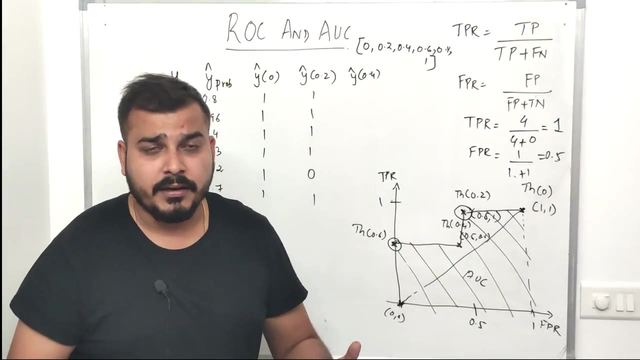 I want high, more higher than this true positive rate. Okay, but I don't care about false positive. then what will happen is that I'll go and select this particular value. in this particular value, I am getting one true positive rate, but There is some amount of false positive rate. but he's saying that I do not care about that, right? 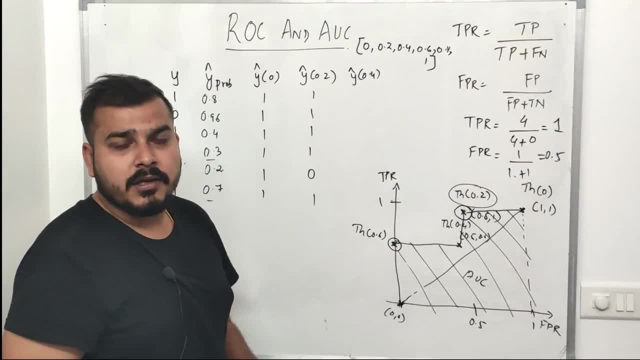 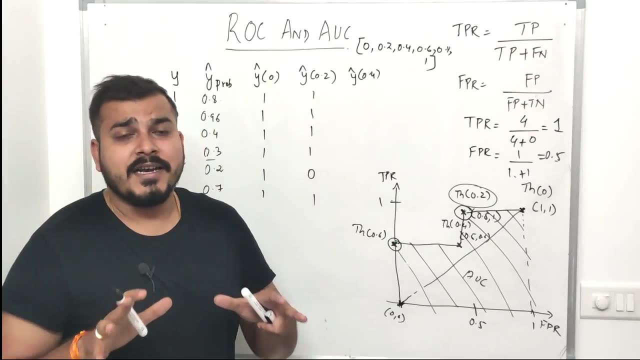 So at that time I can select this threshold values 0.2,. right Now, suppose he says that, Krish, I need to focus on both true positive and false positive. I need to see that particular result. I can also select this one. 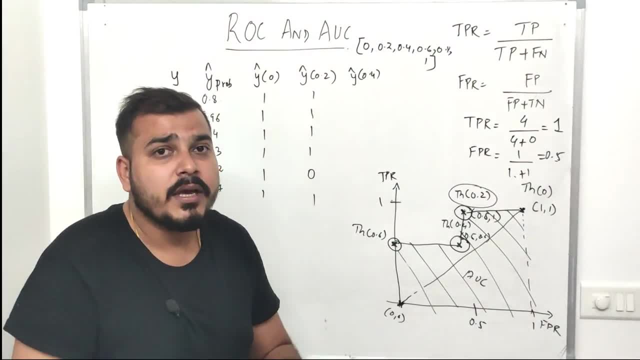 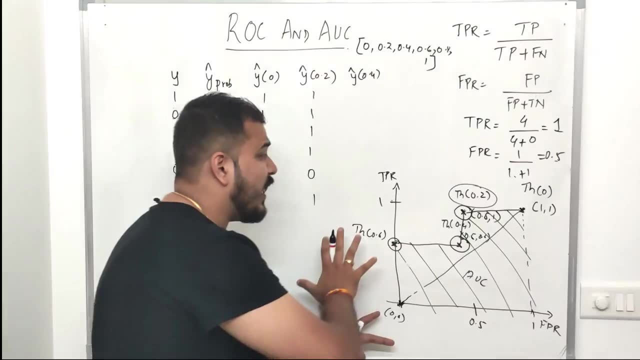 So it depends on the domain expert person, what they are looking at, how your model is actually performing and what is the data that you have represented in front of him. And remember, guys, if you are able to explain him in this particular way, if you are able,